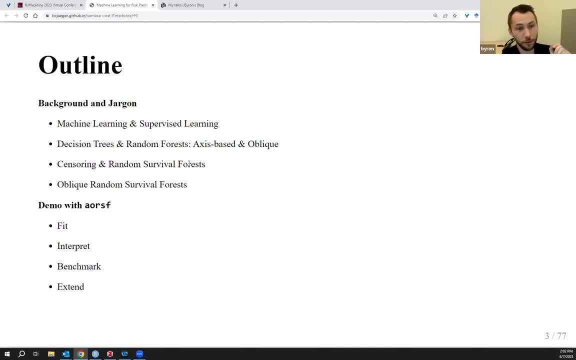 That being said, if this is your first time learning about random forests, I would like to apologize, because this will go too fast and it may seem like too much information at once, but the background section will still be better than no background at all. 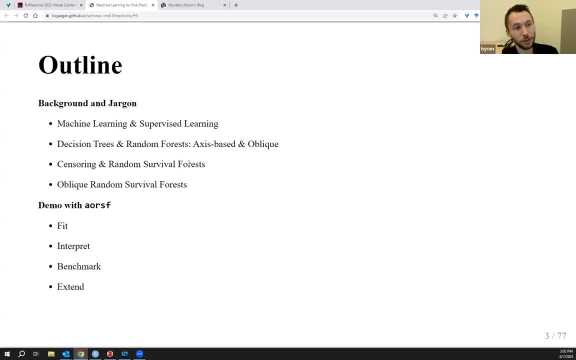 And so once we've covered a little bit of background, I'll transition over to the demo of the AORSA package, Which focuses on Oblique, Random Survival Forests and risk prediction. So we'll be covering how to fit models with that package, how to interpret those models. 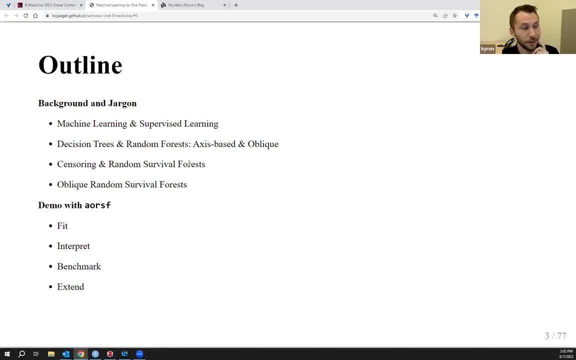 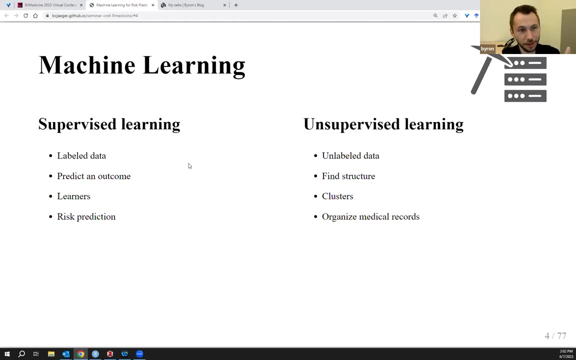 how to run a benchmark, if you'd like to, and how to extend those models for your own tailored purposes and ways that you'd like to grow an Oblique Random Survival Forest. So, starting with the background, we're just going to touch on machine learning, a very broad topic. 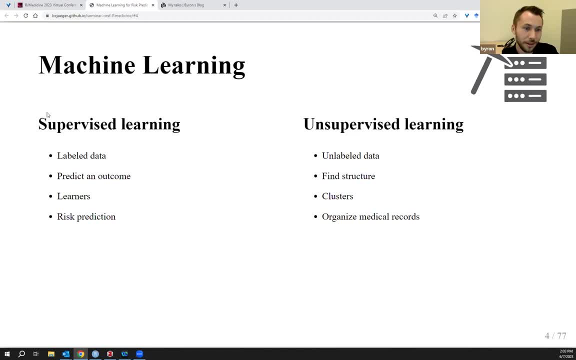 It kind of comes in two phases: There's flavors, There's supervised learning and there's unsupervised learning, and we'll focus on supervised learning today In particular. try and touch on what labeled data is. you know, the prediction problem that we want to focus on, how we engage with that prediction problem, which is learners, and then the specific type of prediction that Oblique Random Survival Forests do, which is risk prediction, which 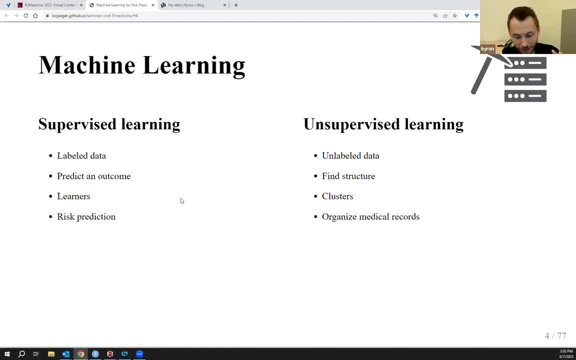 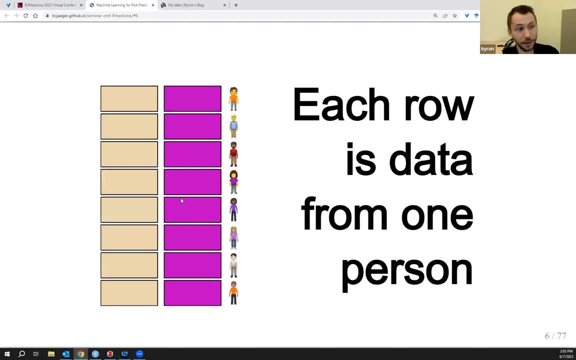 is basically saying we can make predictions for censored outcomes. So we'll try and give the background on all that jargon. All right, so, starting out with supervised learning, we have labeled data. This is a little diagram of a data set and I just want you to kind of imagine each row of this data set. It's giving you information from a particular person and 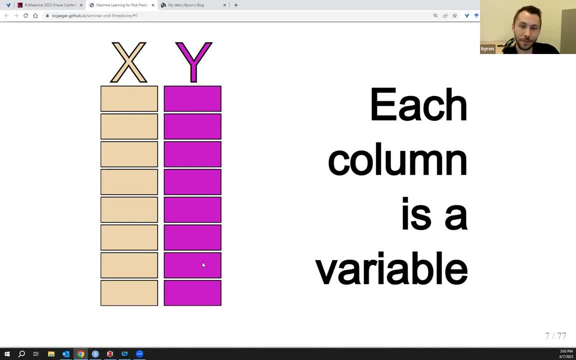 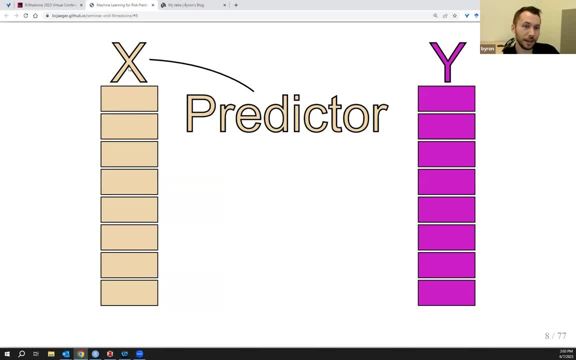 you can also imagine that each column of the data set is a different variable, And so what makes a data set labeled is that some of the variables are designated as predictors- That's what this X variable is here- And at least one variable is designated as an outcome. 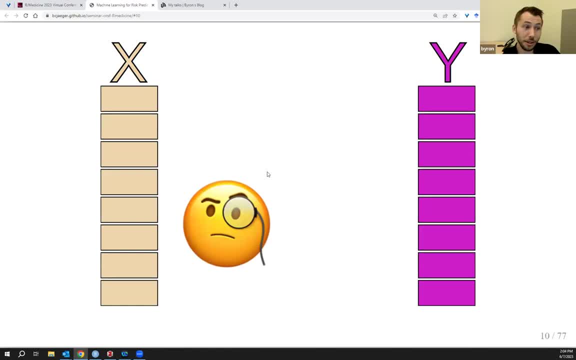 And that's what this Y variable is over here. Usually, predictors are easy to see, easy to measure, they don't require too much money to obtain, and the outcome might require time or might require more money to measure, And so that's kind of why we want to predict the outcome. And so the general problem framework is: you're given the X information and you want to predict the Y information. 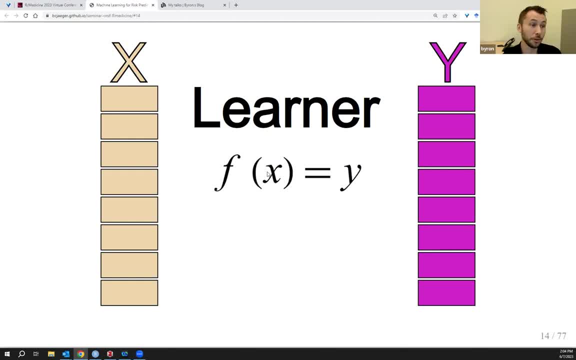 And so the general way to approach this problem is you use a learner. Learner is a jargon term in machine learning and as far as I know, it's just synonymous with prediction model. So if you hear somebody say learner, what they mean is prediction model. 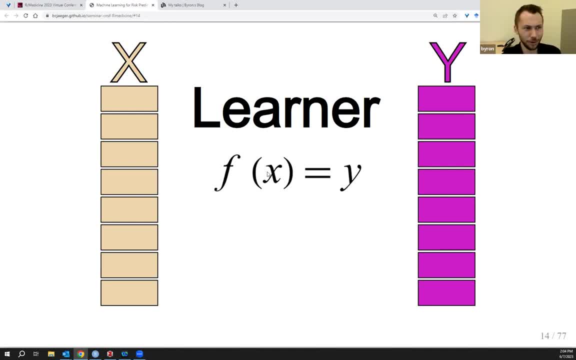 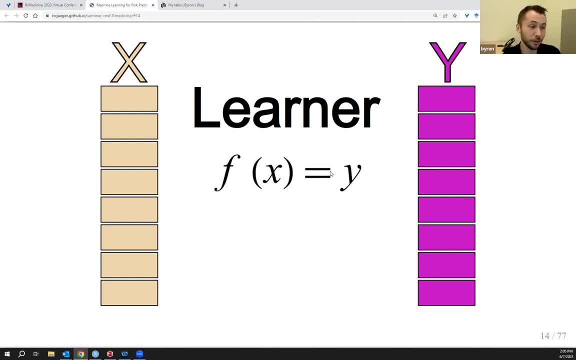 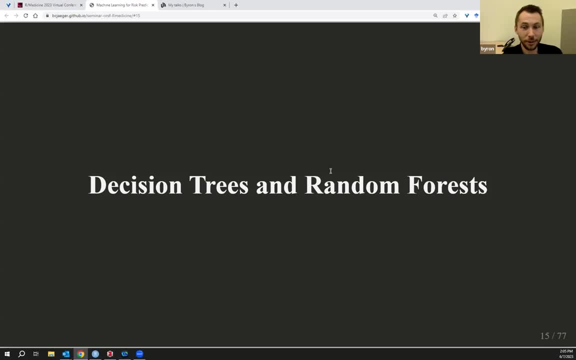 So f is this function that literally maps from X to Y, And we try and estimate that with a learner. Of course, the learner also assumes that this function exists, But that's just a technical background. So now we can talk about two specific types of learners relevant to the demo. 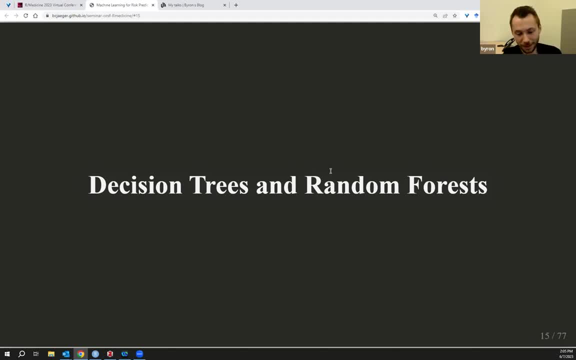 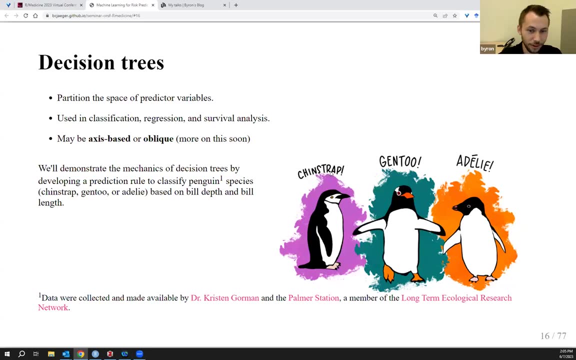 The first is the decision tree and then the second will be the random forest, which honestly is an ensemble of trees or a big set of trees. So first let's just discuss what a decision tree is. Decision trees are a type of learner that works through this mechanism. 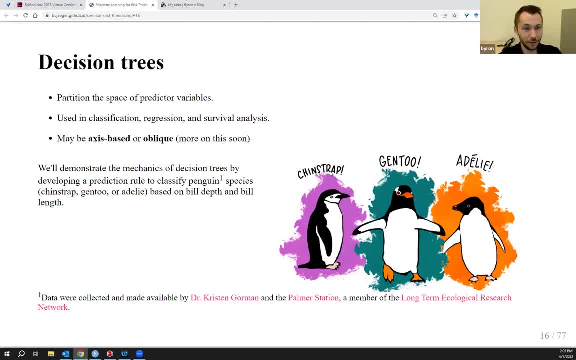 called recursive partitioning, And we're gonna engage with that through some pictures instead of trying to give too technical an explanation. So I'm gonna go through a couple of pictures where we're gonna use a decision tree to do classification of different penguin species. 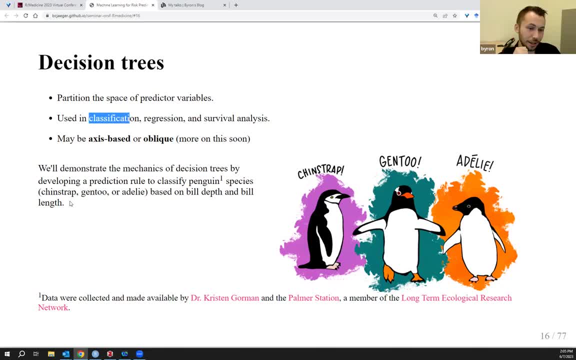 And we're gonna be using this nice data set. It's publicly available, It's very clean and fun to work with. that has chinstrap penguins, Gen2 penguins and Adderley penguins, And so we're gonna try and predict species. 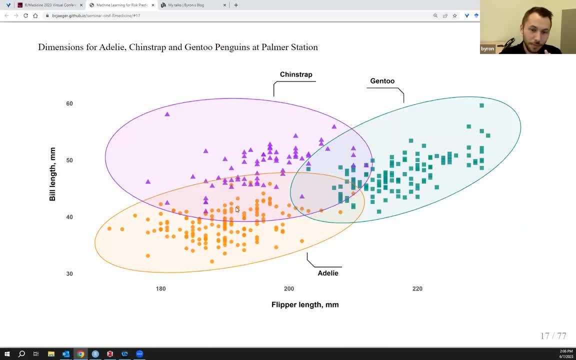 using a decision tree. So this is what the penguin data set looks like. if you visualize it as a function of using flipper length on the X axis and bill length on the Y axis, You can see that in this space there are sort of three different groups. 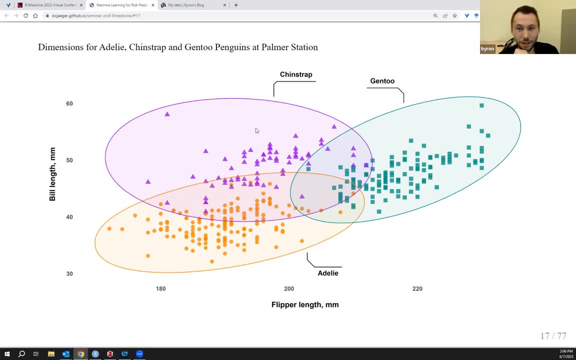 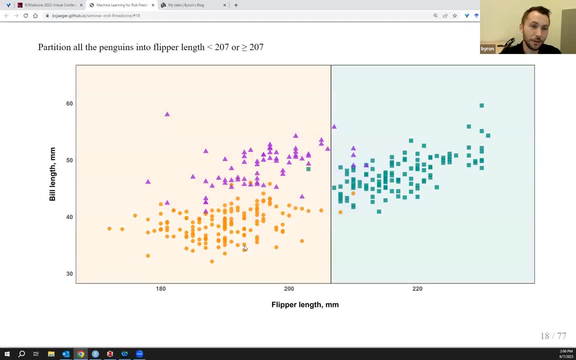 and those groups are kind of the species of the penguins. You've got chinstrap, Gen2, and Adderley here, And if I were to fit a decision tree into these data, it would start by partitioning the data. So what I mean by partition is that it creates two subsets. 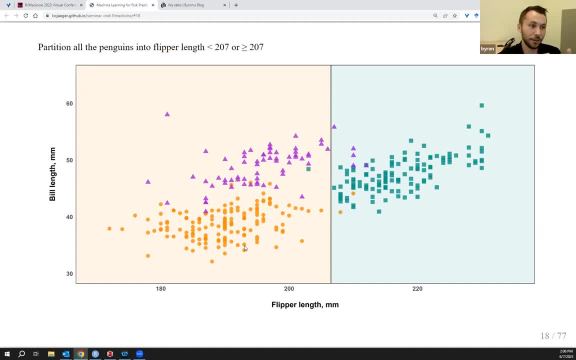 does two subsets at a time And whenever it does this, it creates two non-overlapping subsets that if you put them together, you get back the original space. So here's its first partitioning step. It's created one set on the right and one set on the left. 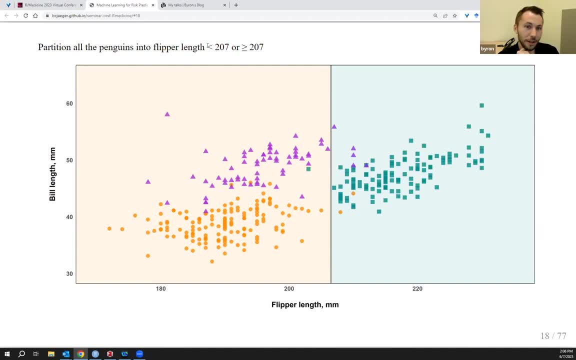 And you can see that it's done this by splitting the data right at a value with flipper length of 207.. And so over here you've got basically all Gen2 penguins. And then over here you've got all the Adderley penguins. 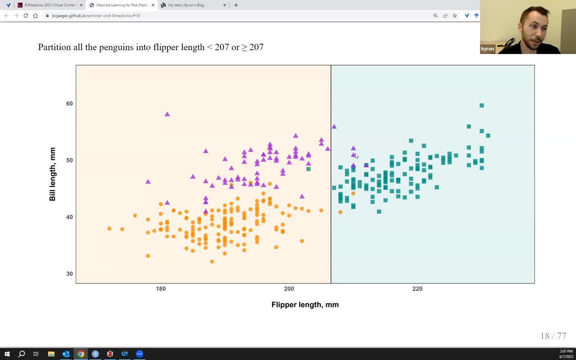 and the chinstrap penguins, And so the reason that subset works like this is that the decision tree tries to maximize the difference between the two subsets it's creating in terms of the expected outcome. So the expected species on the right-hand side is clearly Gen2 penguins. 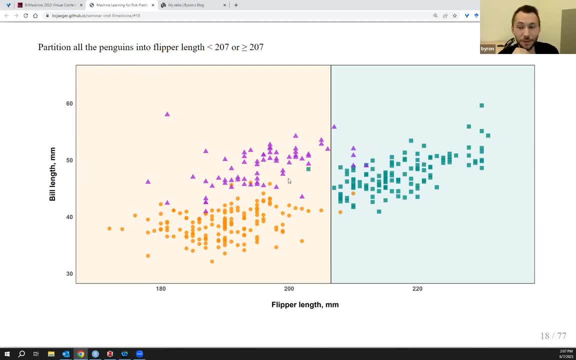 And on the left-hand side, it's clearly not Gen2 penguins, And so if I were to allow the decision tree to grow another partition, this is what it would come up with. Now. it's partitioning based off bill length, but only on this left-hand side figure. 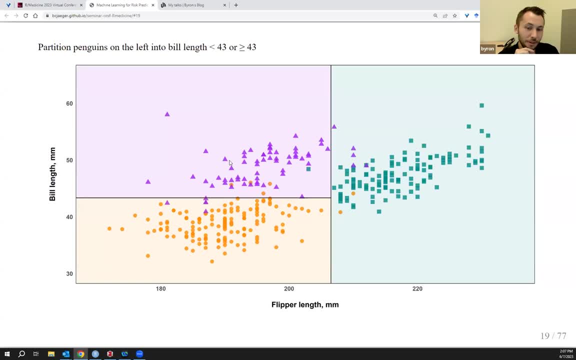 And the bill length cut point is 43. So now in this subset up here on the top left you can see it's purely almost nothing but chinstrap penguins, And then down here it's almost nothing but Adderley penguins. 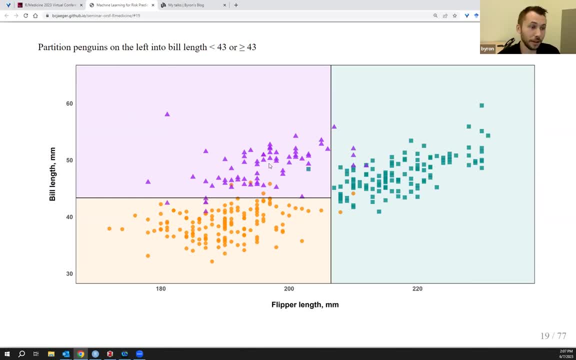 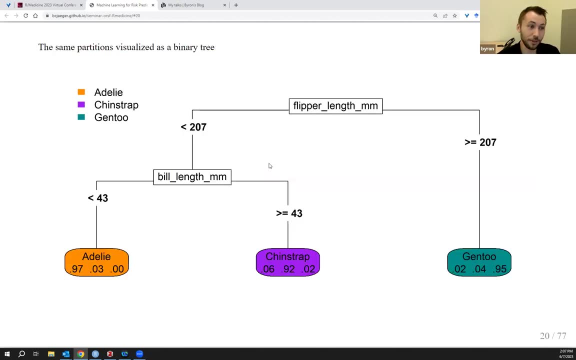 So these three regions are called leaves in the decision tree, which isn't immediately clear why it's called a leaf, But when you draw this, the same graph now can be visualized as a binary tree And you can see that these regions at the bottom. 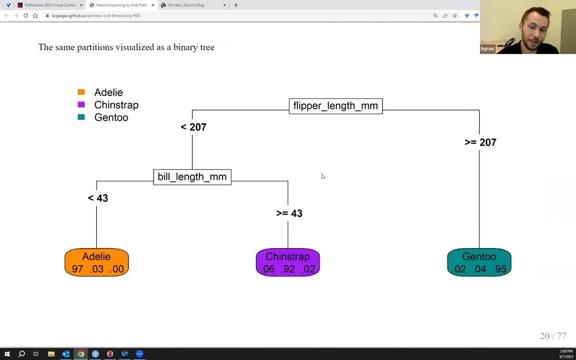 are essentially just the three regions that are shown here. Now you can kind of see why they're called leaves, Although this is a tree that's been flipped upside down. this is the formulation of a tree. that is the reason why people call it a tree. 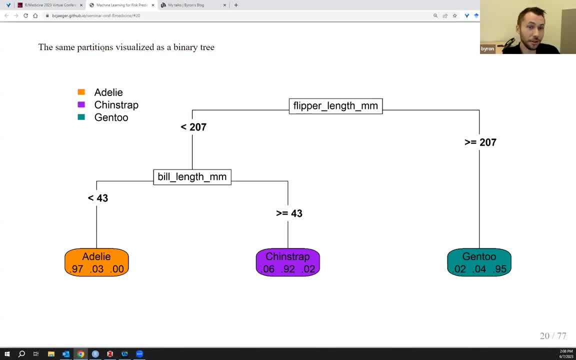 So if you want to compute predictions with a decision tree, the idea is that you can't just start at the top of the tree with whatever data you're trying to predict, And then you follow the instructions until you get to an ending point, a leaf in the tree. 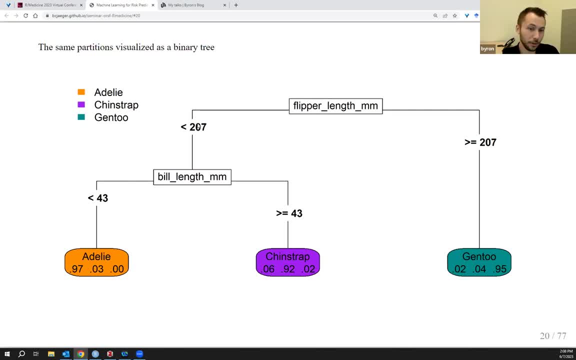 So let's just say that we started out up here and our flipper length is less than 2.07.. So we come down here And our bill length is- I don't know 50. So we end up in this leaf. 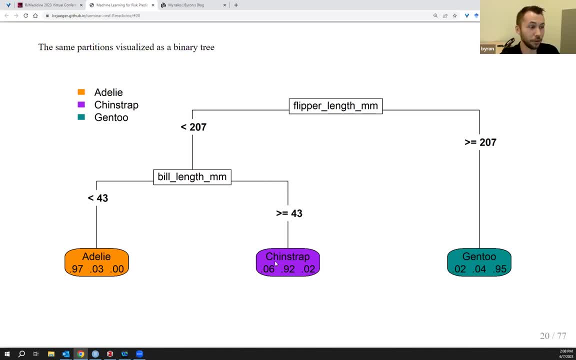 So now our predicted value is going to be given to us by the leaf in the tree, So the predicted species is chinstrap, But the actual predicted probabilities are listed out here. So we have a 6% predicted probability of Adelie. 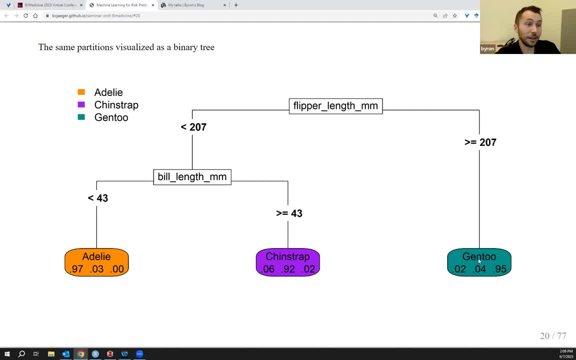 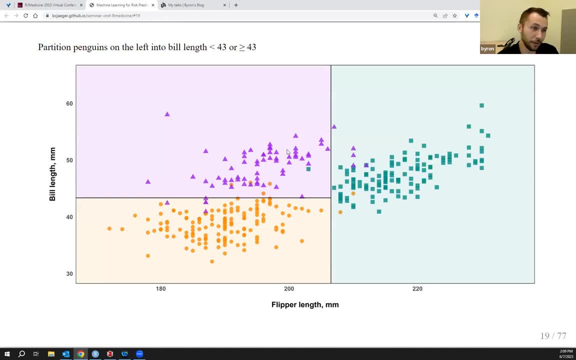 92% of chinstrap and 2% of Gentoo. And in case you're wondering why that is, this is the leaf that we ended up in And you can see in this leaf 92% of the training data that were in this leaf from the tree. 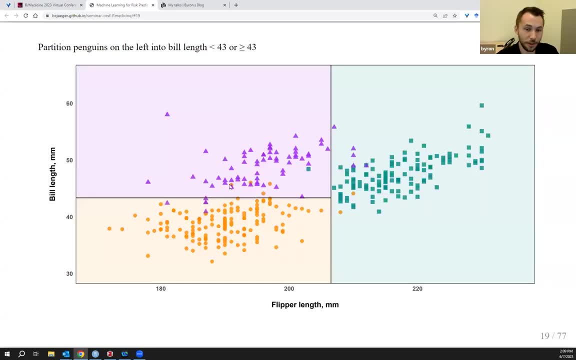 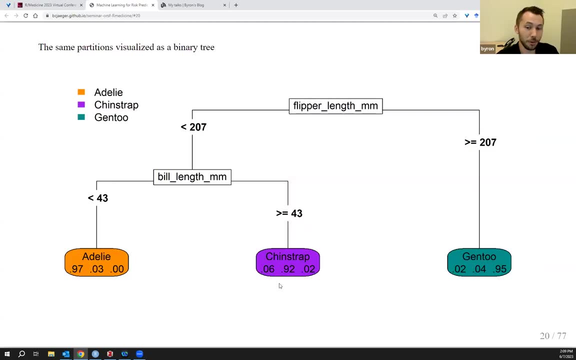 is fed were chinstrap pigments: 6%- these three dots here were Adelie pigments- And 2%- this one dot here was Gentoo. So the predicted value of the leaf is basically just a summary of the training data that we're. 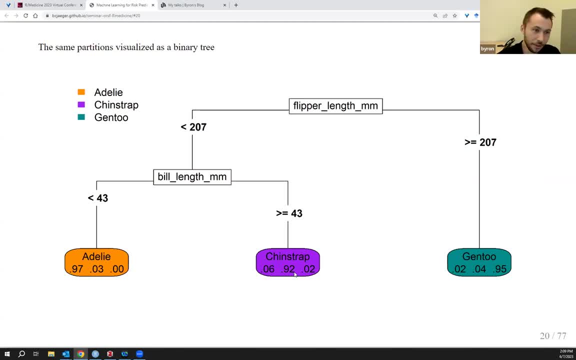 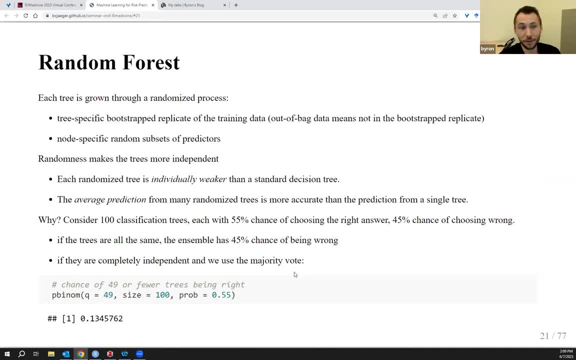 going to use to make sure that we're able to get the right answer in that leaf when the tree was grown. So this is the basic mechanics of a decision tree, And now we're ready to talk about the random forest. So the random forest is a big set of decision trees. 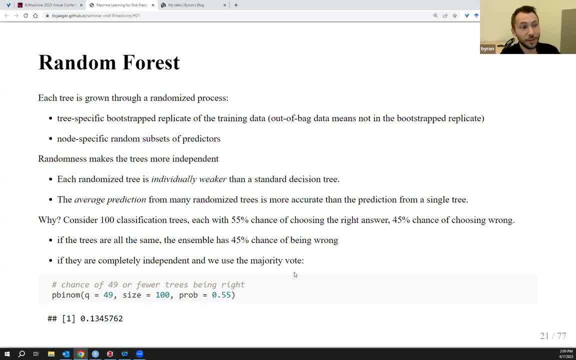 It works like a committee. When the random forest wants to make a prediction, it gets a prediction from all of its decision trees And then it does something to kind of make a majority vote or average them together or take some summary of the predictions. 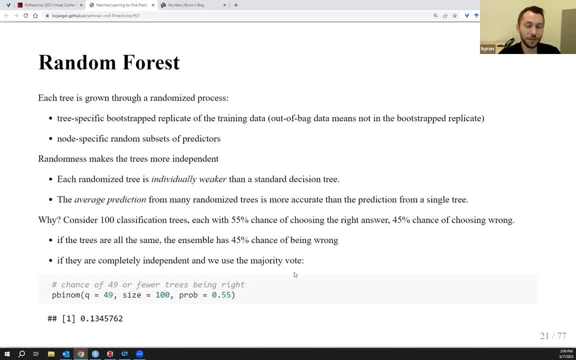 from the decision trees. So what makes the random forest a little interesting is that it grows the trees with a little bit of randomness. And it's a little counterintuitive, because when you grow trees with randomness you actually make the individual trees less good at prediction. 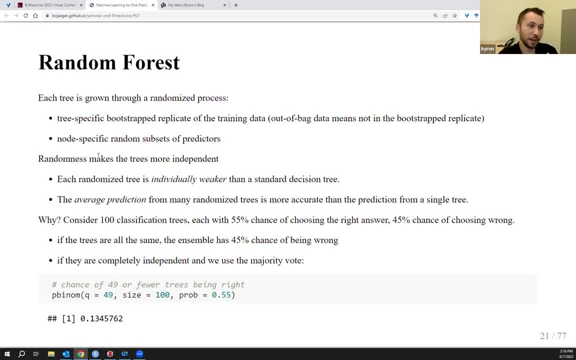 But you make each tree more independent from the other trees. So, to get into a little bit of detail, what actually is randomized when you grow the decision trees in the forest is you get tree-specific bootstrap replicates of the training data. So you start with your training data. 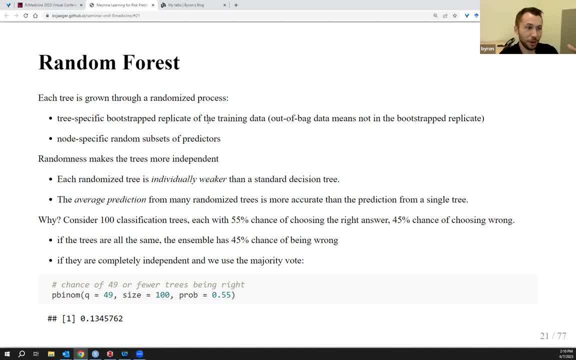 and you just take a bootstrap subset of it, which gives you about 63.2% of the original data in your bootstrap subset, And then you have a little bit of data that's not in the bootstrap subset, which is called out-of-the-bank data. 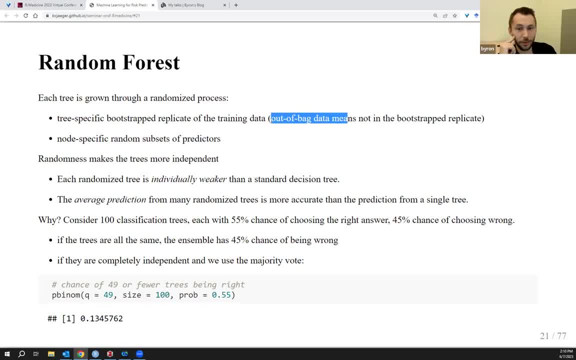 And this concept will come back up when we talk about the stuff in the demo. So I'm just putting the seed in there, And then you also have random subsets of predictors being used. Every time you have a tree, you're going to have a tree. 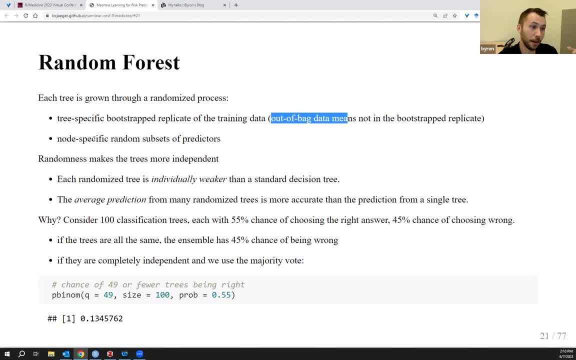 And in the end you're going to send to that tree the tradingemplo, which is right in front. So the center- sagtion comes from the tabular. So we really just have to break it into two pieces and then what we do with our data is. 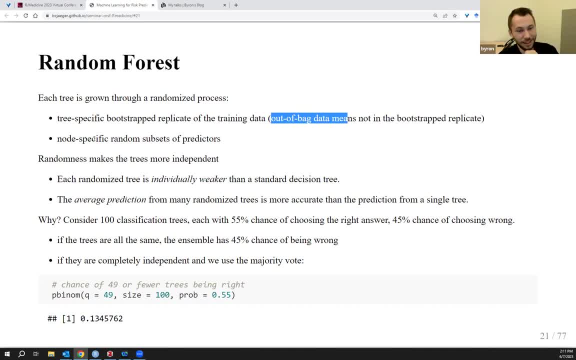 we take that data and we run it through the lassen, economics as that tool, And once we do that, the data will phase out and eventually죠 the decision. trees in the random forest grow two new branches, So randomness will make the trees. 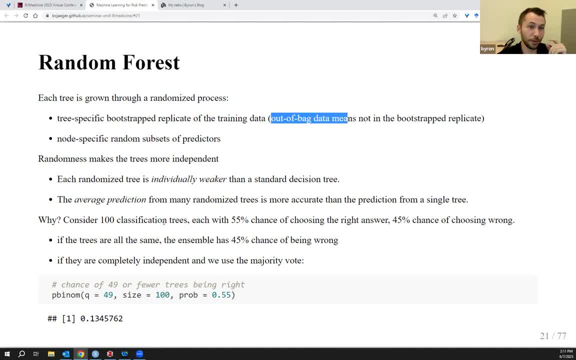 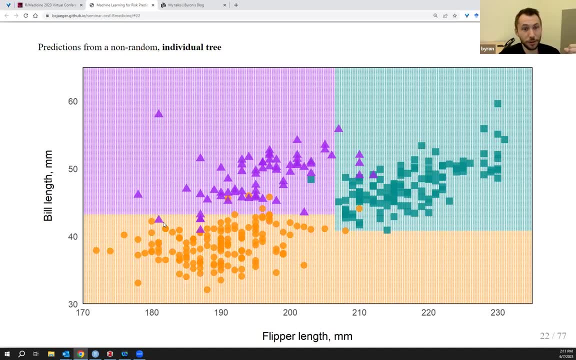 more important, more independent, But it also makes individual trees weaker of time. But I also can show you with some visualizations how a random forest does a really nice job of computing predictions. So here you can see some decision boundaries from a standard. 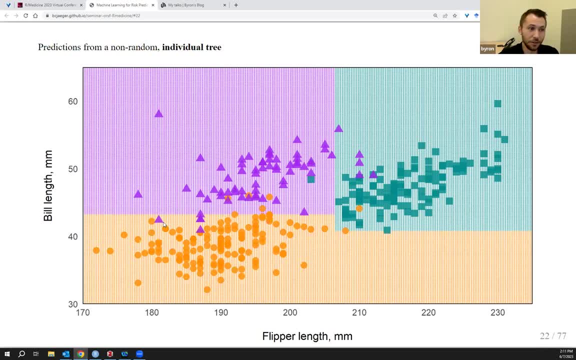 non-random individual tree, and it does a nice job of predicting our pigment data. Now I'll show you what a decision boundary looks like from a tree that has been grown with this randomization and it actually does a little bit worse job of creating a decision boundary here. 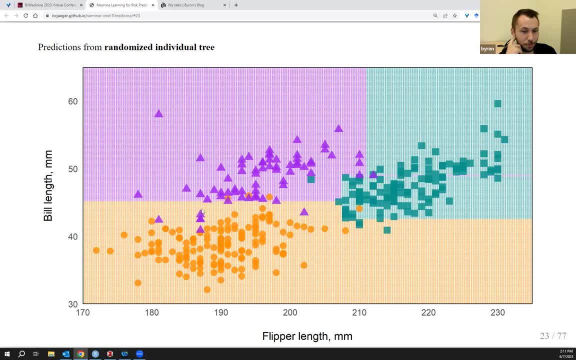 because you can see that it's not quite correctly classifying these purple points, whereas the original decision tree did. And the reason this randomized tree isn't correctly classifying those points is probably because those points weren't included in its bootstrap replicate of the training. 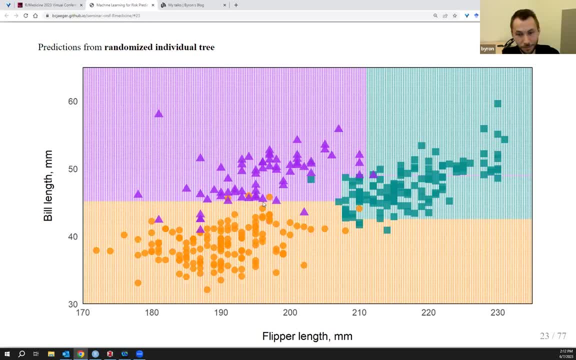 data so it didn't even see those points when it was being grown. Now I'll show you the decision group's randomization. So this is a randomization tree and it's not quite correctly classifying the decision grid from the random forest. So this is an ensemble decision grid. It's just taking the 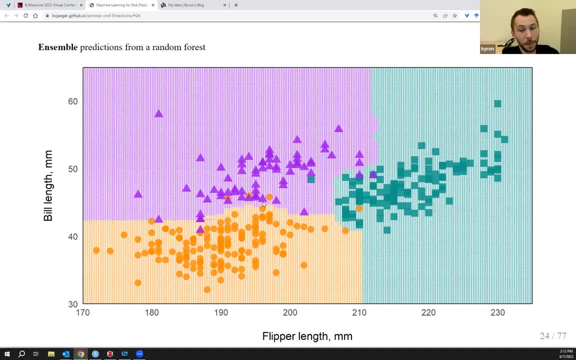 predictions from all of the trees, all those randomized trees that it's grown, averaging them together. And what's surprising is that it does such a good job. The decision boundary looks very in tune with the data. It doesn't seem to be overfitting. I can see somebody has joined and is. 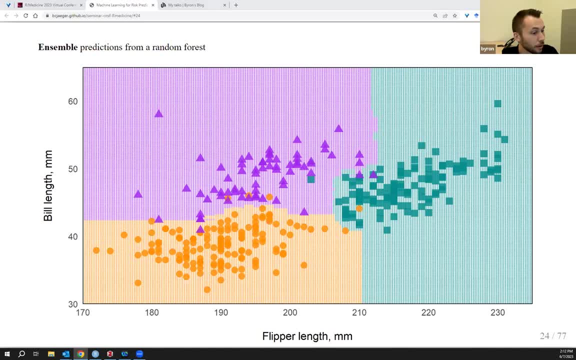 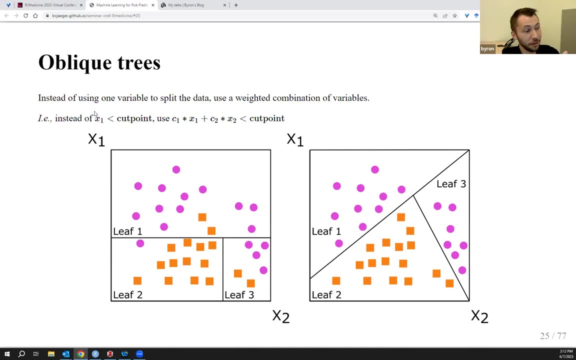 asking about a link to the content, so I'm going to put that in. Thank you for joining, by the way. So now let's just touch on what no-blink tree is. We've kind of covered the basics of decision trees, And decision trees can be either axis-based or oblique. An 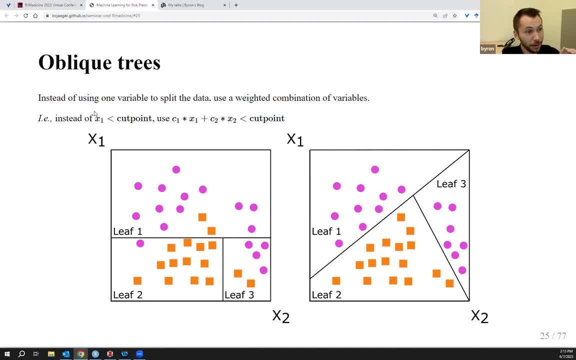 axis-based tree is going to be drawing these lines in our predictor space that are perpendicular to the axis that the predictor that we're splitting on is, And so you can see, an axis-based tree will kind of make splits like this And you have, for example, a tree that's split in half and then 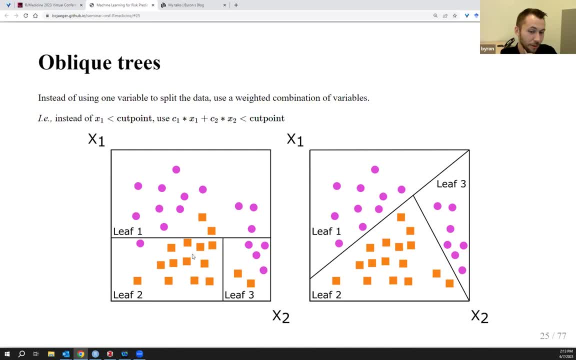 you have these lines that are drawn perpendicular to the axis of the predictor, And an oblique tree is different from an axis-based tree because an oblique tree uses a weighted combination of predictor variables instead of using a single predictor variable when you partition data. So 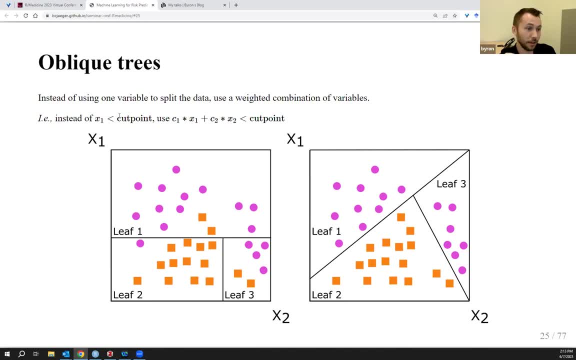 instead of using x1 being less than some cut point as a splitting mechanic, we actually use something like a constant times x1 plus a constant times x2 is less than a cut point, And this leads us to get decision boundaries that look like this. So I'm going to show you a couple of examples of this. 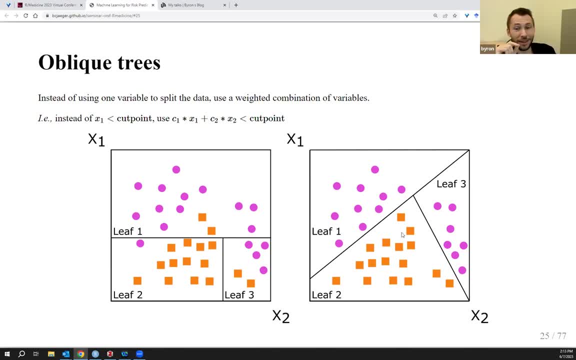 We have oblique decision boundaries, because these boundaries that you're seeing are neither perpendicular nor parallel to the axis. All things considered, I'm not the biggest fan of the term oblique. I don't know what the right name would be, though, so it's just what we call it, And so when? 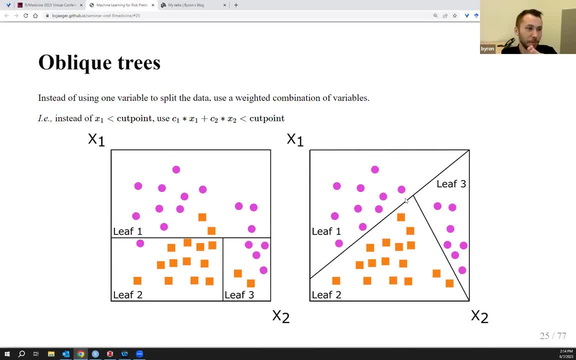 you hear the word oblique, you can just think like: oh, these are more flexible decision boundaries because we're using linear combinations of variables to make splits instead of just a single variable. And so when you look at the decision boundaries from an oblique tree, you can see how the 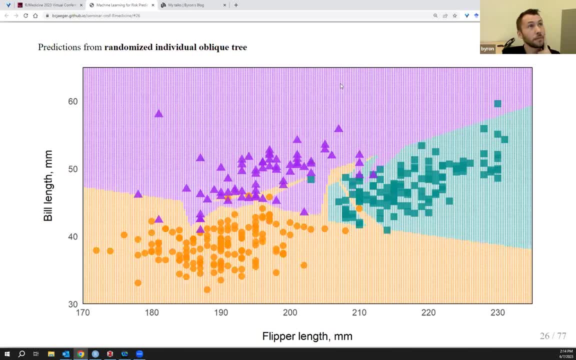 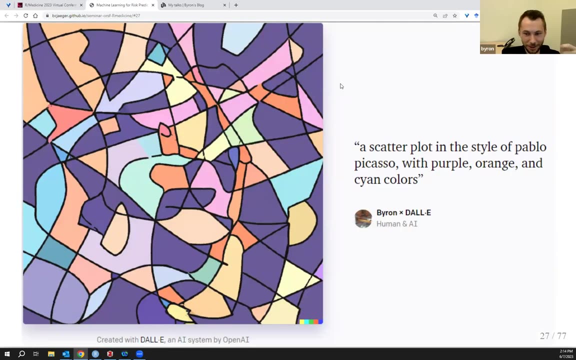 boundaries are no longer perpendicular to the axis that we're splitting on, And you may also kind of think to yourself like, oh, this is kind of maybe like what a decision tree would look like if Pablo Picasso had designed it, And I was curious about this. I wanted to go over to Dolly the 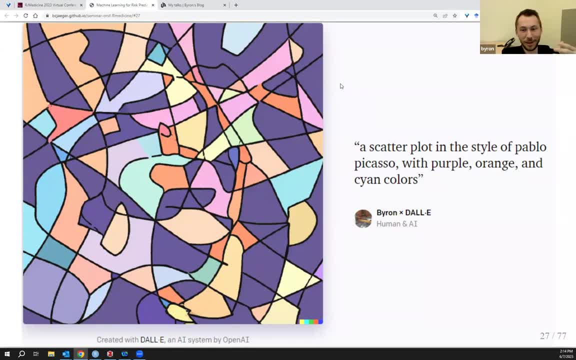 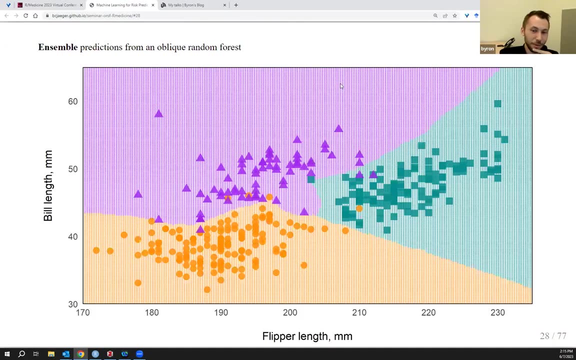 AI image generator and see if it would give me back- you know, basically an oblique decision tree, decision boundary, if I typed it in like this, like a scatterplot in the style of Pablo Picasso, And in my opinion it's pretty similar, Pretty similar. So, but what's really neat is that when 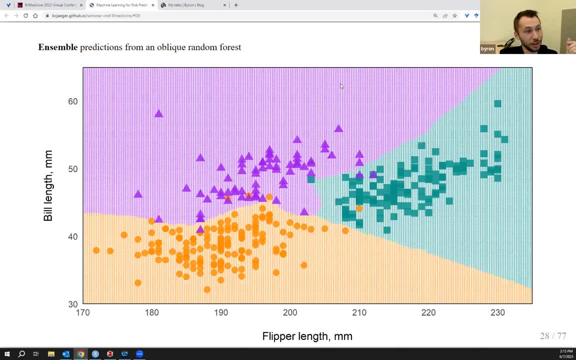 you ensemble a whole bunch of predictions from oblique trees, you get back a decision surface that looks very reasonable, very smooth. In fact, this is the big thing that distinguishes axis based trees from oblique trees. Oh, I see a question. 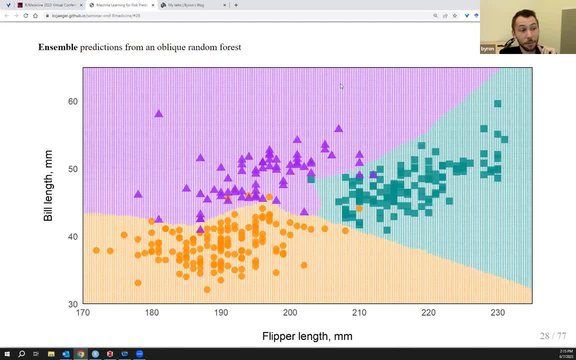 in the chat about linear subspace trees. I'm not the biggest expert on those. I'm not gonna dive too far into it because I'm not an expert and also because I don't wanna eat up my whole hour with, like some other topics. 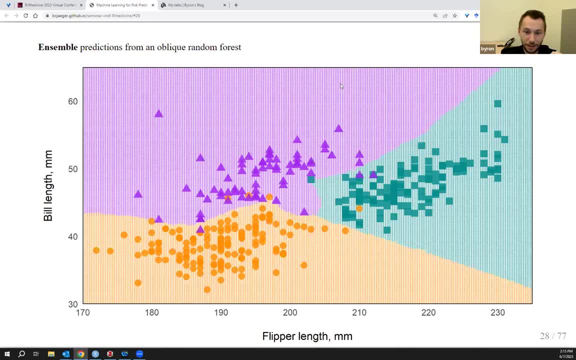 But I'm gonna pivot back over to the slides. So the decision boundary that you're seeing here is a lot smoother than the axis-based one, And that has a lot to do with the fact that the decision boundaries for the individual trees are not perpendicular to the axis. 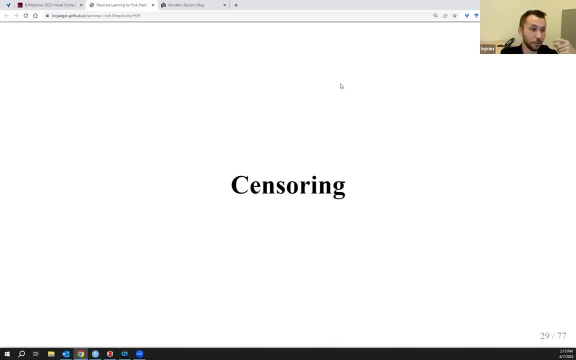 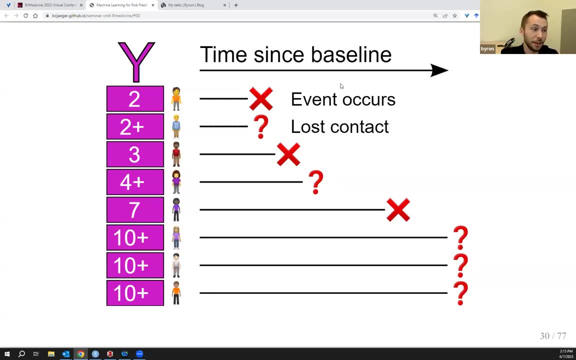 So another thing to consider is sensory. This is why we have to talk about risk prediction instead of just straight probability prediction. So sensory means that we have incomplete data about the outcome, And this happens when you may start a study and you may have an outcome. 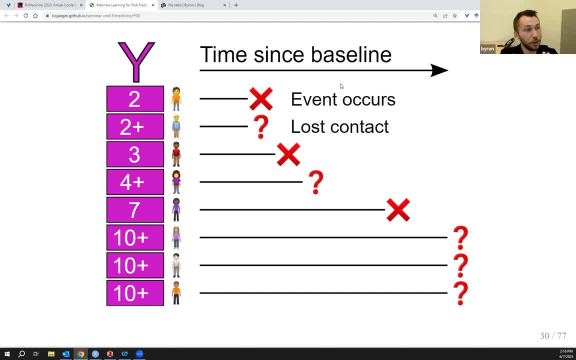 like the development of, let's say, hypertension, and you just wanna follow people and see when they develop hypertension. So it's like a time to event framework. So over the course of the study, which, let's just say, the study lasts 10 years. 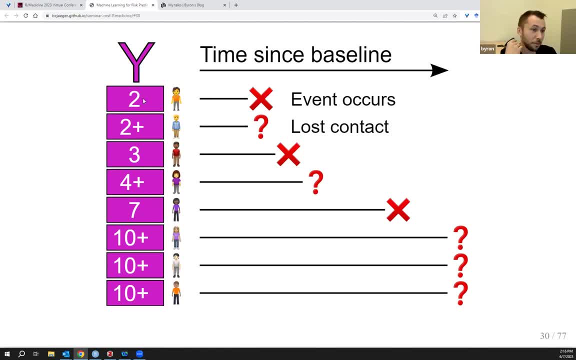 you're gonna have some people who have the event and they might have the event before 10 years collapses. So this is here's somebody who has the event at two years. But then you have other people who decide that they don't wanna be a part of the study anymore. 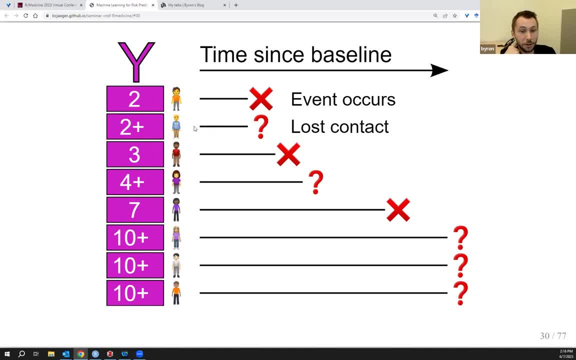 So they drop out or you just lose contact with them And you don't know they don't have the event up until the point where you lose contact And so you really don't know if they have the events during the 10 years or not. 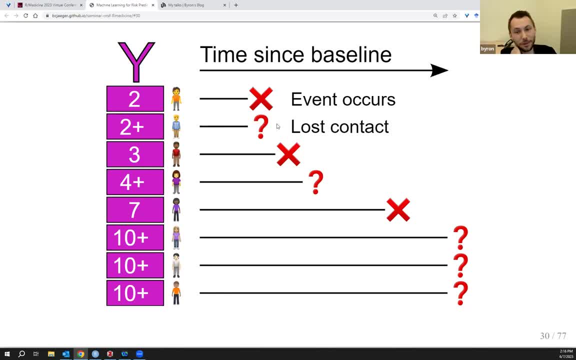 And so this is what we have to deal with when it comes to computing predictions. Oh, I see that the speaker sound is echoing a lot. I'm not quite sure why that is. Is anybody else getting that audio feedback? So echo in the room? 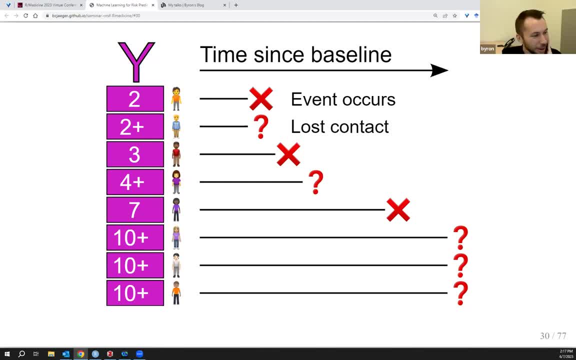 Well, just okay. Okay, I guess I'll continue. It seems like it's good enough, So anyway. so if we were to be asked the question of can we predict risk in the next two years for hypertension, we could theoretically use this person's data. 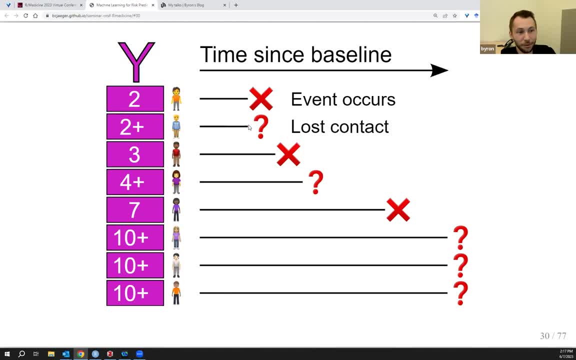 because we know that they don't have hypertension in the first two years. But if we're asked to predict risk in the next five years, we have to be very careful about how we use data from somebody who was censored at year two Because we wouldn't wanna assume. 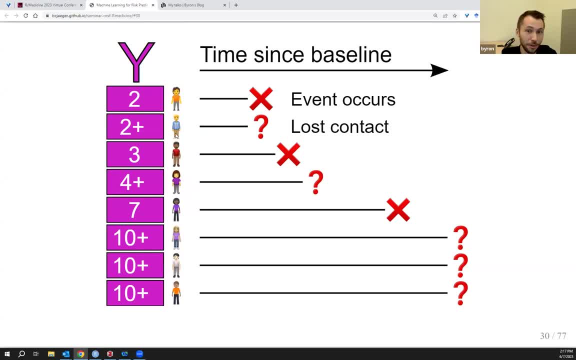 that they didn't have the event for the three years that we weren't in contact with them. So this is where risk prediction comes into play and not to go too far into the details. but we have to be very intentional about how we use sensor information. 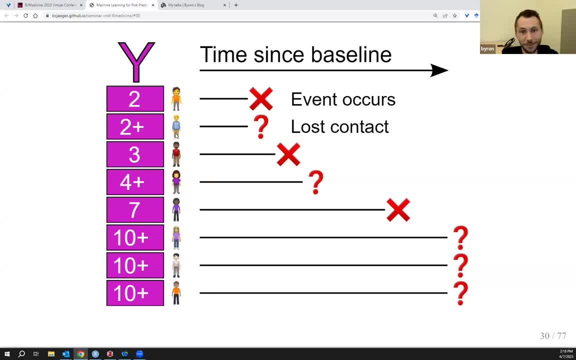 so that we don't bias our predicted probabilities of the event happening. So with risk prediction, we just have to be aware of the fact that we wanna make a prediction about the event occurring in specific time span, And we have to sort of specify what that time span is. 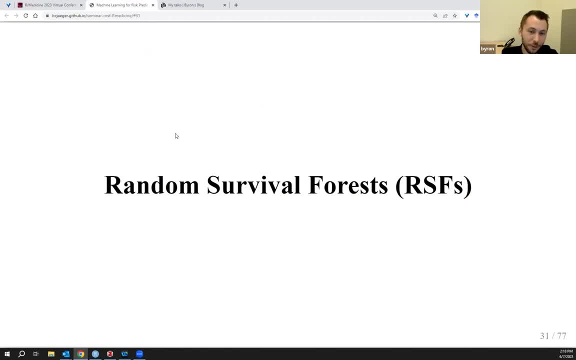 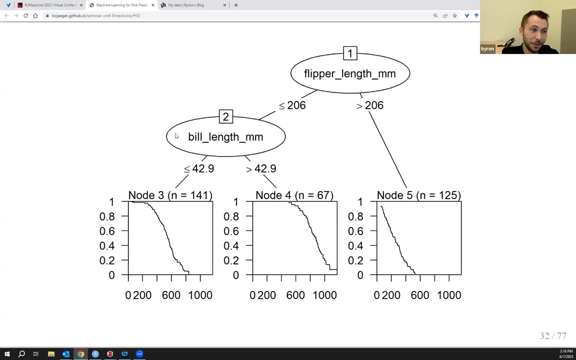 All right. so this is where random survival forests come into the mix. Random survival forests are designed to deal with censored outcomes and they can give you risk prediction, So the way that these work is that they're basically just the same as any other. 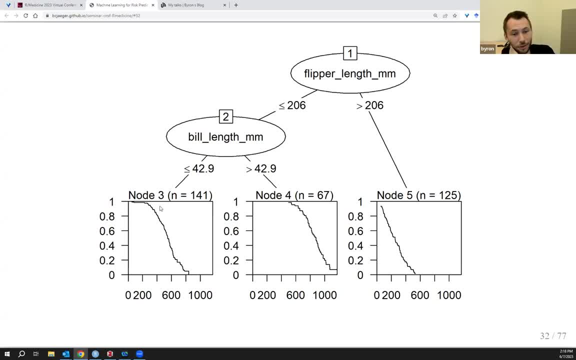 their trees are the same as any other decision tree, but in the leaves of the tree we fit Kaplan-Meier curves- basically predicted survival curves- to the training data that are in that leaf And this is how we can get predicted risk. 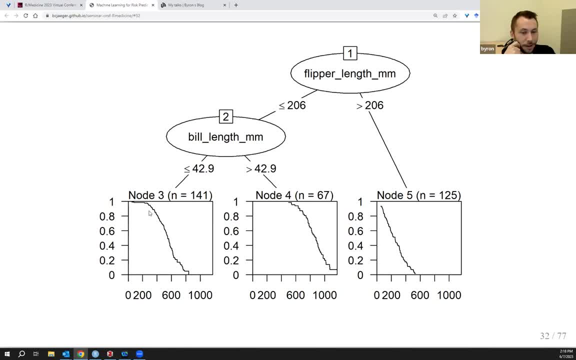 Somebody will give us a time right. So if we get a time of 200, we go into this node and we see a time 200 about. you know, all of the observations in this node haven't had the event yet, And so that's how we can get these predicted probabilities. 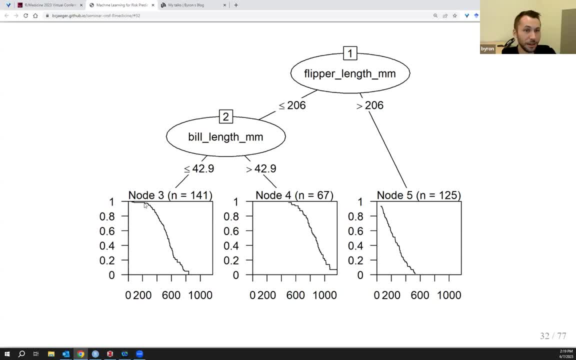 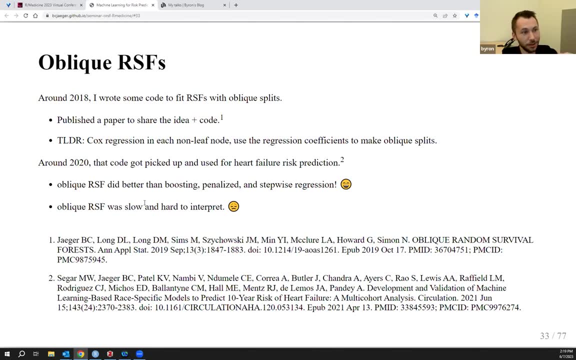 at specific times, And then we aggregate them in the normal way and we get an ensemble prediction from the forest. All right, so now we can put these concepts together and talk about the model that Amaris fits, which is the Oblique Random Survival Forest. 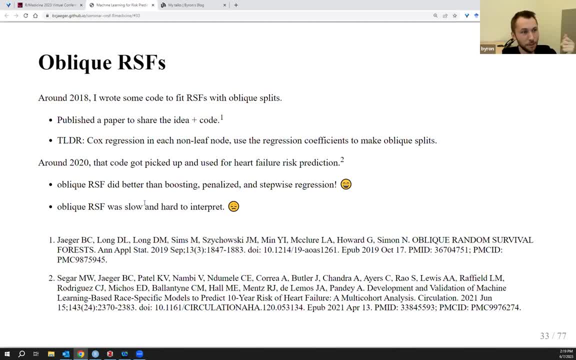 The background of this is that I wanted to fit an Oblique Random Survival Forest back in 2018.. I couldn't find code to do it, So I wrote something a little rough and I thought it worked well enough. So I wrote a paper and I wanted to share the idea. 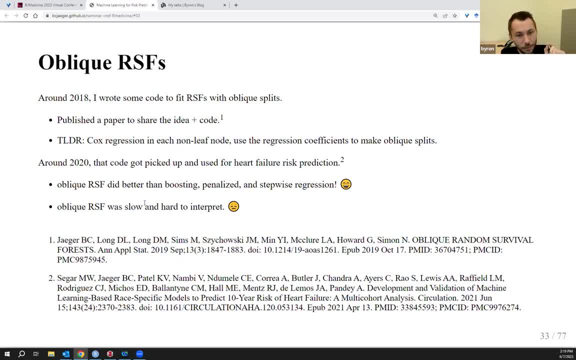 and also share the code. And the basic idea was, while we're growing the tree, we'll just kind of fit a Cox model to the data in each decision node and then use the predicted values from that Cox model as the linear combination of predictors. 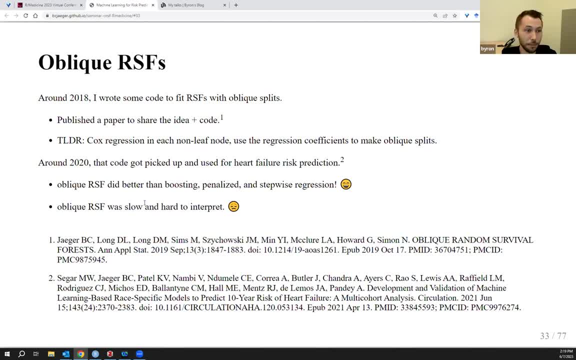 And that works okay. It ended up being pretty good at prediction and a general benchmarking test. So around 2020, the code that I wrote was picked up and it was used in a separate study to develop a heart failure risk prediction model. 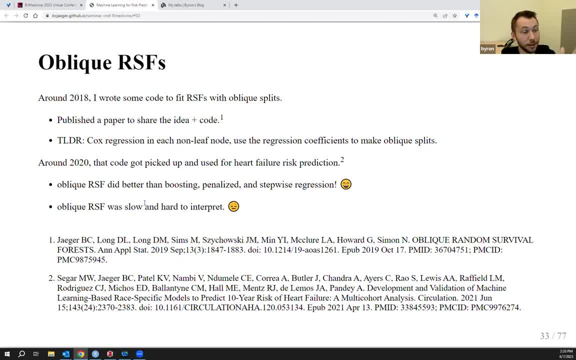 And the Oblique Random Survival Forest did well in that study, which was very exciting. but it also helped me realize, as I was watching the person I was collaborating with, that I was actually using my code And they had trouble And, of course, they didn't complain about it. 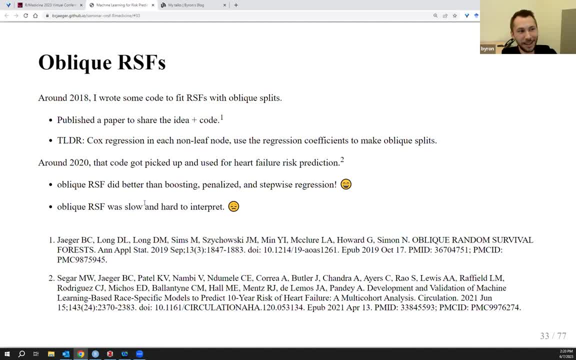 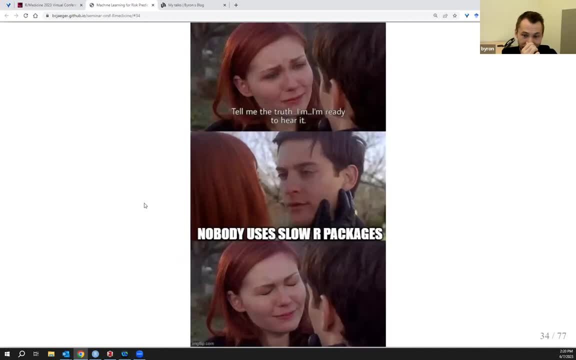 or anything like that. but I was able to see that my code was becoming a bottleneck in their analysis because it ran slow and it was not as accessible as I would want it to be, So I decided after that that there was this sort of rule. 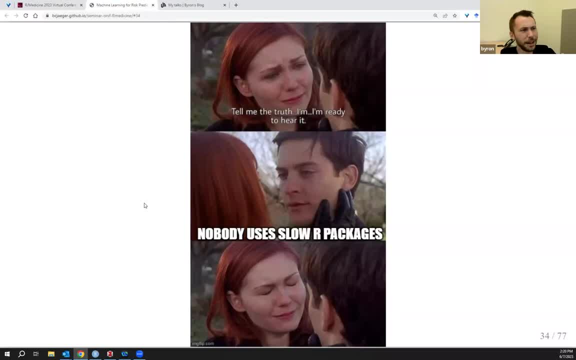 in the R universe that I wasn't quite aware of. There are a lot of really good R packages out there, but if you kind of look at the R packages that are used most frequently it's the ones that are fast. The fast R packages really have a lot of traction. 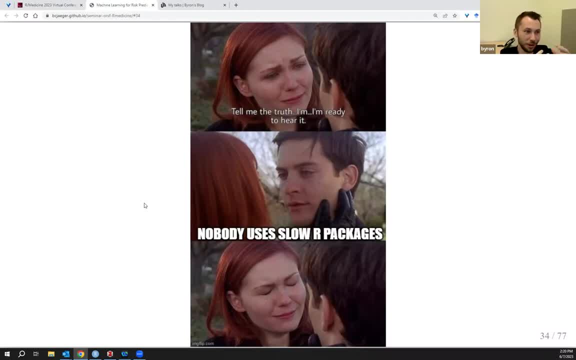 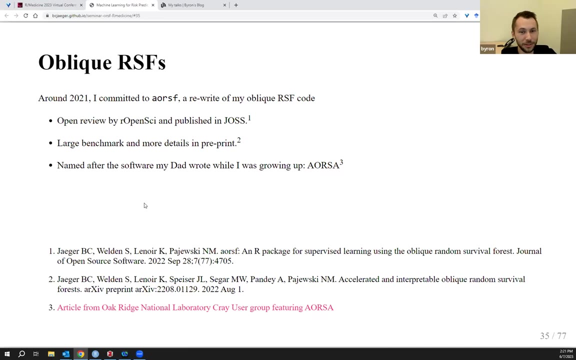 And I don't think that's a problem. I mean, having your work run fast and allowing you to make adjustments, updates and tune things is good. So I realized I needed to rewrite my code and come up with ways to make it efficient. 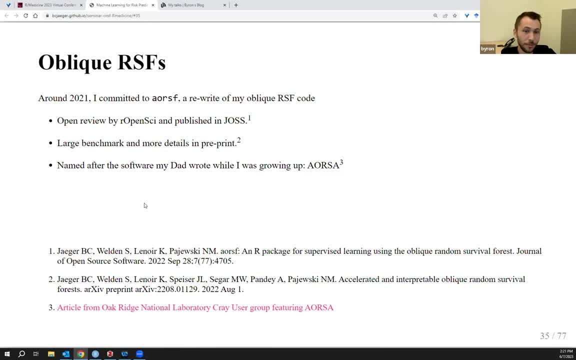 and a lot more accessible for users. So I went through this process. It's been a while, but I rewrote my code and I made it into a new R package called AORSEF. It went through a review process by ROpensci. 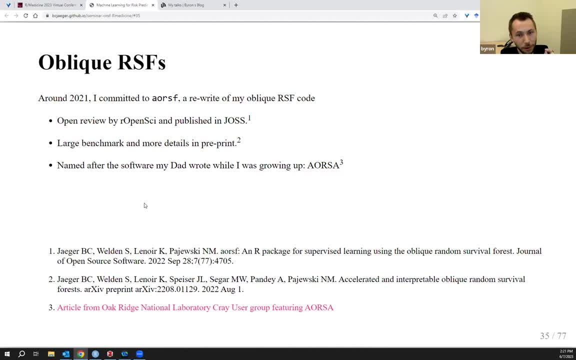 which I found extremely helpful, And it was published in the Journal of Open Source Software. That's what JOS stands for right here, And I ran a much larger benchmark on it to kind of understand how good it was at making predictions. The benchmark is currently just sitting on archive in a preprint. 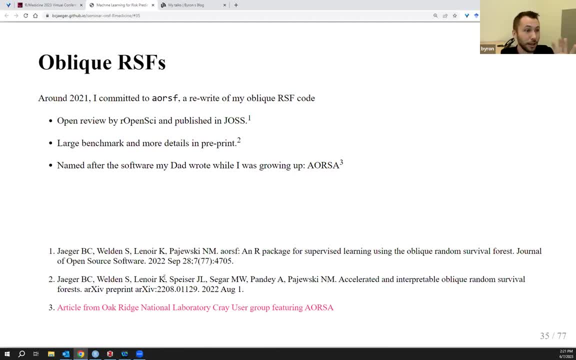 I invite you to go and check it out, Thank you. It's lots of details and a lot more details than we'll get into here, But it's hopefully pretty comprehensive And as a bonus, I renamed the R package AORSEF. 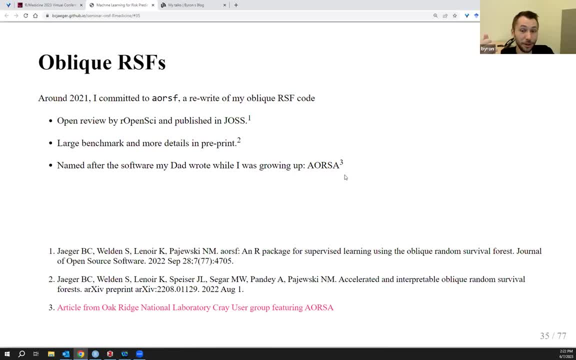 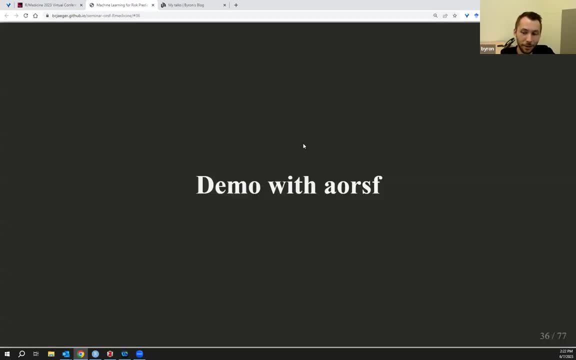 because a long time ago my dad was developing his own software. He called it AORSA, So I thought it would be kind of funny if we just basically shared the same acronym. So this gets us to the point now where we can start doing the black demo. 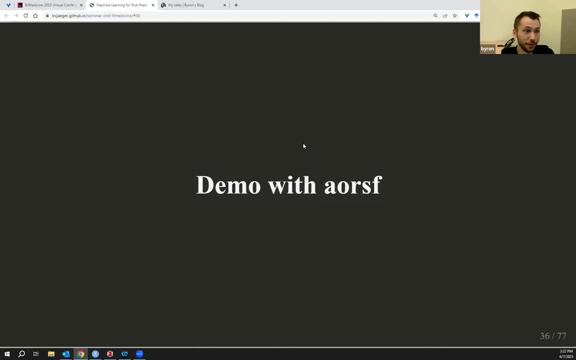 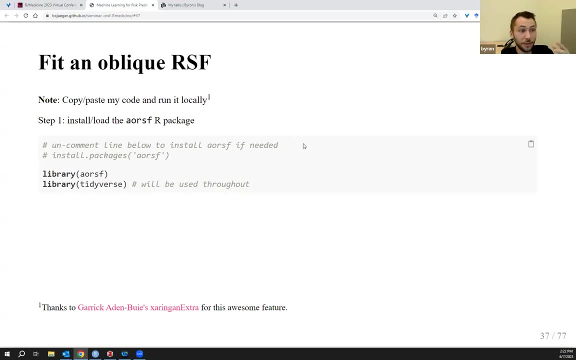 I hope the background was helpful. It definitely was a fast. It was a fast race through all the topics, But now we can at least have a little bit of shared vocabulary, And so here we can start. The first thing you might want to do is install AORSA. 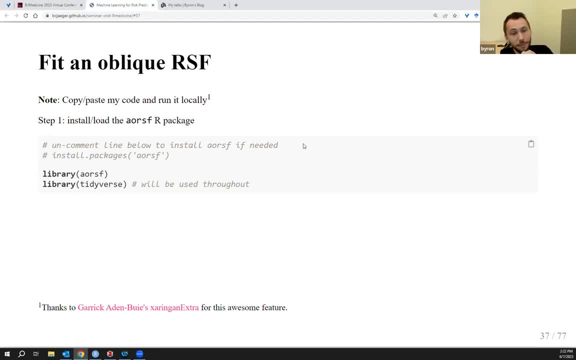 To do this. you can run installpackages, because AORSA is on CRAM And now I'm just going to point out you can run these. You can open these slides up on your computer. The link to the slides is in the chat. 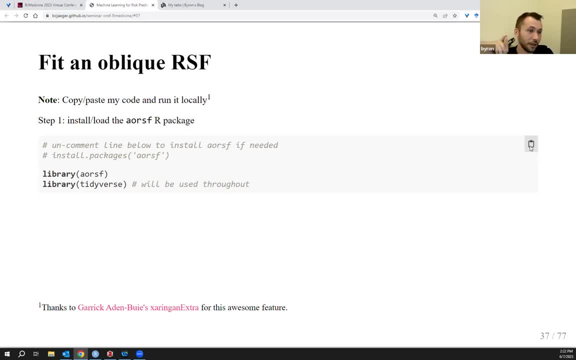 And then, when you have it open, you can click On this little button on the right-hand side of any of these code blocks And it'll automatically copy the code. And so then you can come over to an RStudio session and just kind of paste the code in. 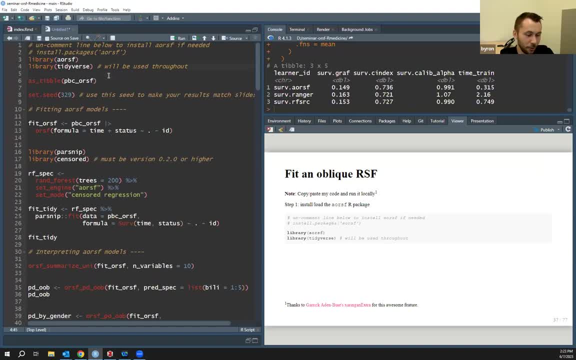 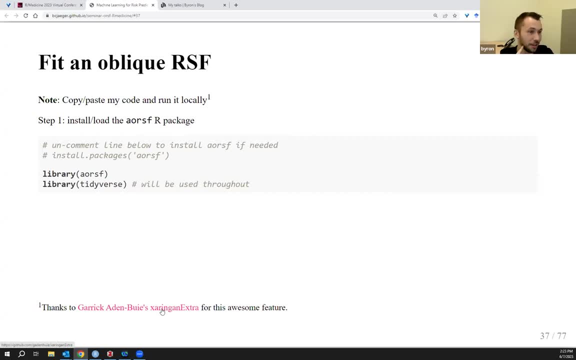 And I hope that will be a nice, convenient feature for folks to use. This is a really nice feature brought to you by the Schrodinger extra package, by the way. So you're going to want to have AORSA downloaded And you're probably also going to want to have a tiny burst. 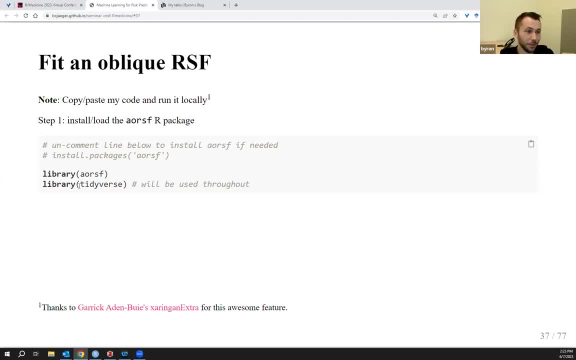 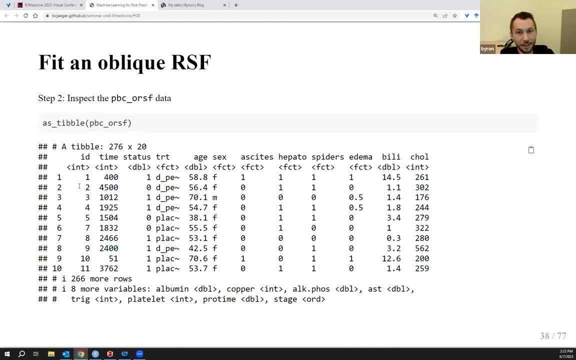 We'll use the tiny burst kind of throughout to just do things, And a next step in the demo will be to briefly look at the data that we're going to be modeling. So there's a data set in the AORSA package called PPC AORSA. 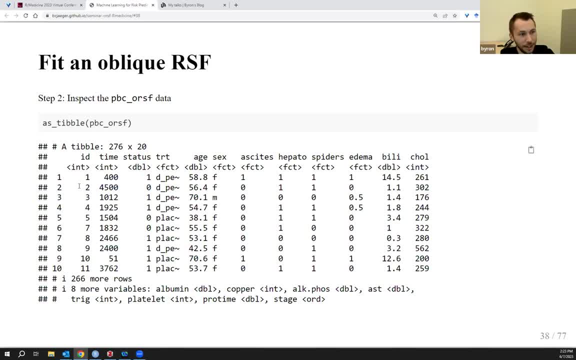 It's a very slight modification of the PPC data from the survival package And you can see when we look at it. it's got 276 observations, 20 columns. One column is in the ID That's not going to be used for prediction. 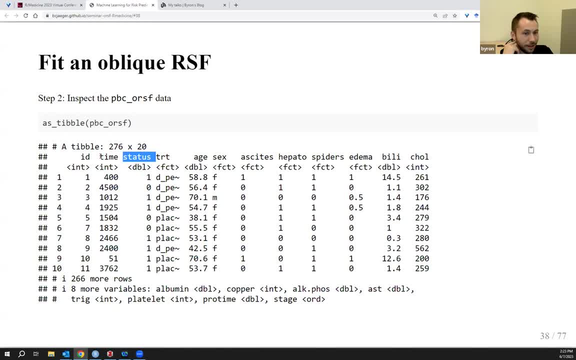 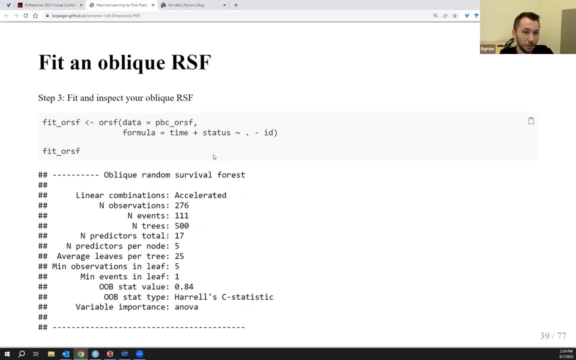 And we have a time column and a status column. These are the time until the event, and then whether the event happened or whether the person was censored, And then we have all these other columns that are potentially used as predictors. So now we're ready to fit in. Oblique Random Survival Force. 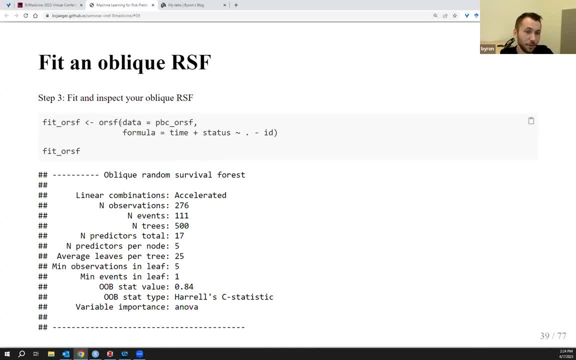 And to do this, we use this function called AORSA, And it's only going to require two things: It requires a data set and it requires a formula, And you'll see on the next slide, there's actually a number of different ways. 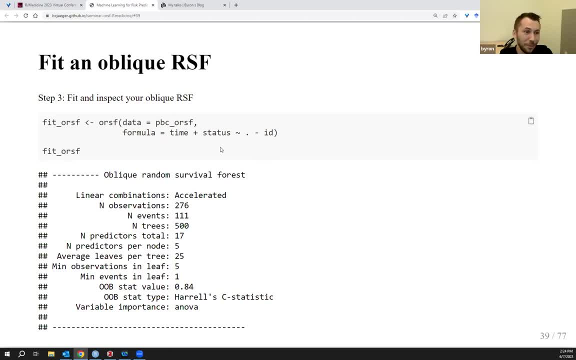 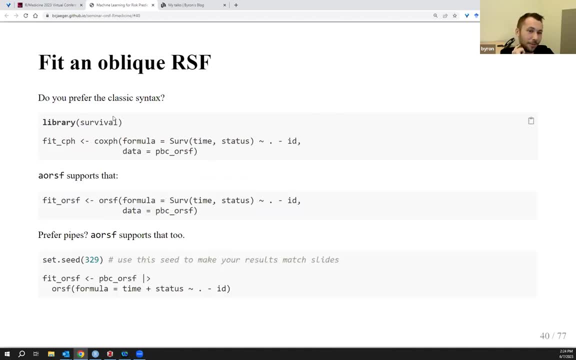 to specify the formula because I want to let people use the syntax that they like. So we'll come over to this next slide. If you are a long-term R user, you've probably used CoxPH at least once And you'll know when you use CoxPH. 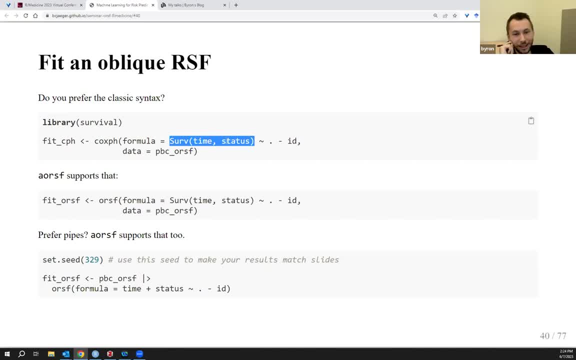 you specify the outcome with this serve object, So it's capital S serve, and you put the time variable in and then the status variable, And you can do that if you're using AORSA. There's no need to use this time plus status syntax. 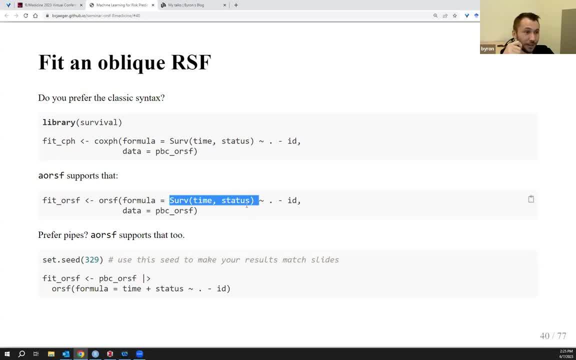 unless you like it. You can also specify your formula using the standard serve object And then you can use most of our formula shortcuts on the right-hand side, And what I'm showing you here is you can use this dot shortcut. That means: give me all the predictors or give me 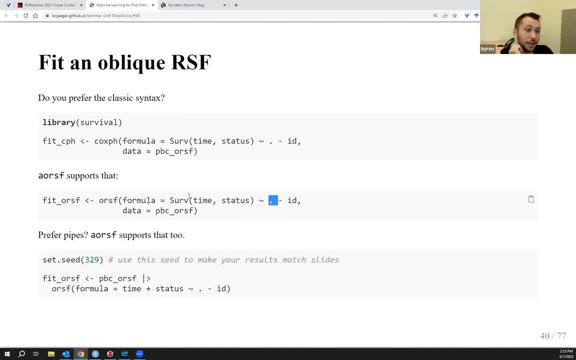 all the variables in my data set that aren't on the left-hand side of my formula. And then you can also use this minus sign to say except for this predictor. So our formula here means give us all the predictors except for stuff on the left-hand side. 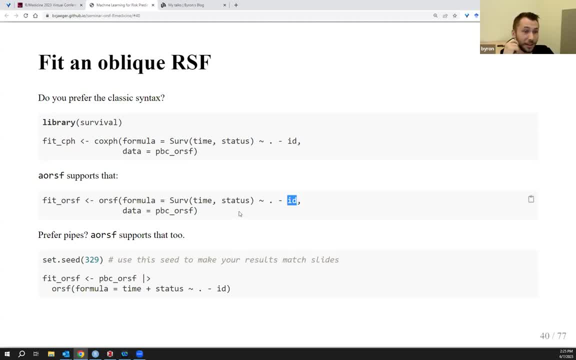 except for this predictor called ID, because we don't want to use the ID as a predictor. And then, of course, we just specify the data after that. So a couple of different ways. you can specify models with the AORSA function. 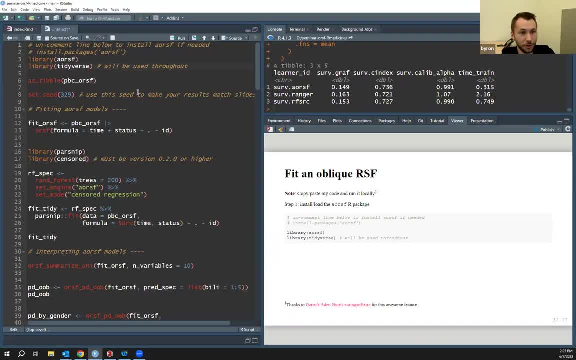 And now I'm just going to flip over to RStudio for a second to kind of walk through how this code will run. I'm setting my random seed to be 329 in case you want to get the same fit as me, And I'm using the AORSA fit right here. 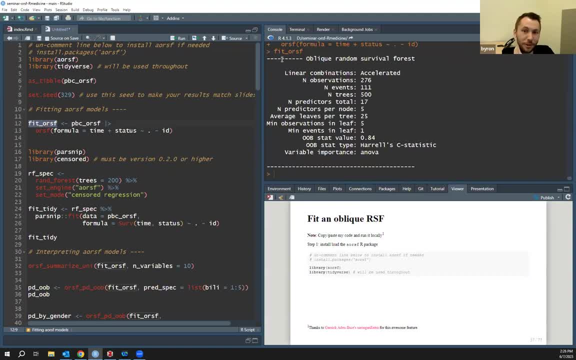 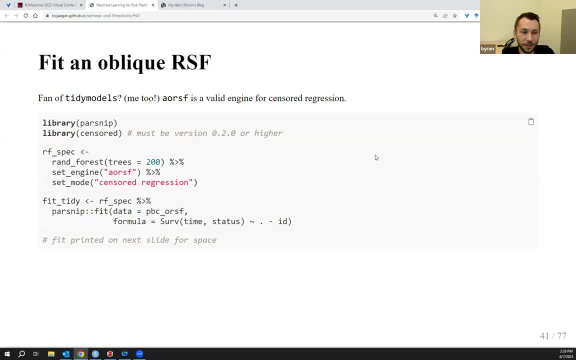 And so I can just print it out. You can see the printout comes in a similar syntax to the random forest SRC package Back over here. If you like, you can go back to the slides. So also, if you like using tidy models, I'm right there with you. 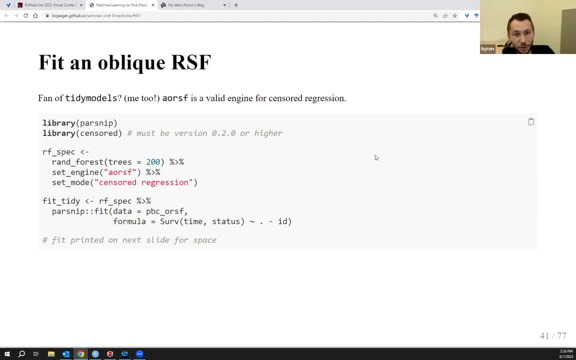 I think tidymodels is a very nice set of R packages, And so, as of version 0.2.0, in the censored package you can now select AORSA as an engine. So if you wanted to set up a modeling pipeline with tidy, 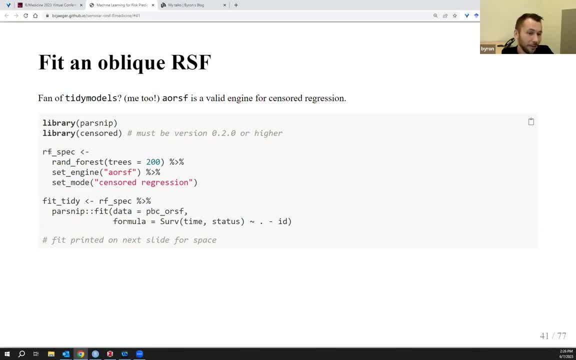 models and you wanted to use AORSA. this code is kind of how You specify a random forest and then you set the engine as aorsive and then you're going to have to set mode to be censored regression, because that's all that aorsive currently does. 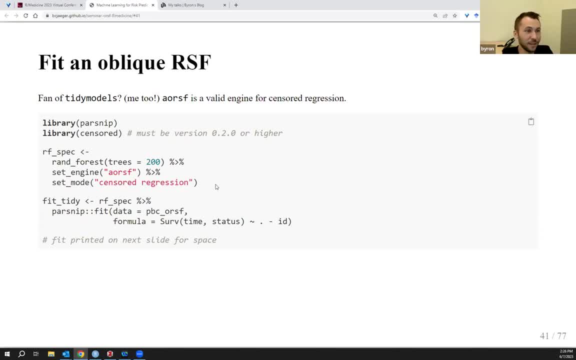 I do think it'd be great to make it work with classification and standard regression as well. I just need to set aside six or seven months to sort of do that. But once you have that random forest specification set, you can then go ahead and use the parsnip fit function to fit an aorsive model. 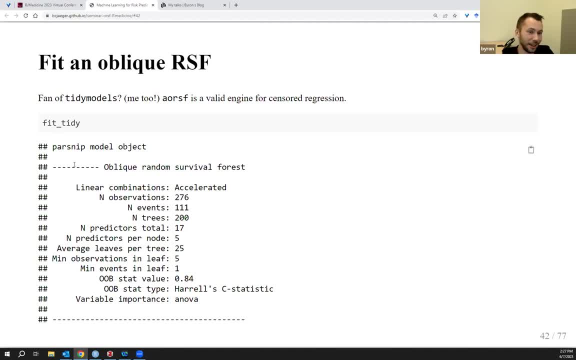 And you'll see, it's just now. you get the same printout, you get the same aorsive model, but now it's wrapped up in the parsnip modeling attributes. So it's a new addition to the tidy models universe, and I'm excited to see how the censored package evolves, because I think that they're doing work on that. now to 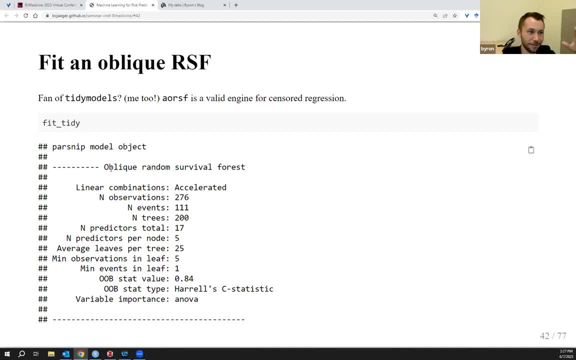 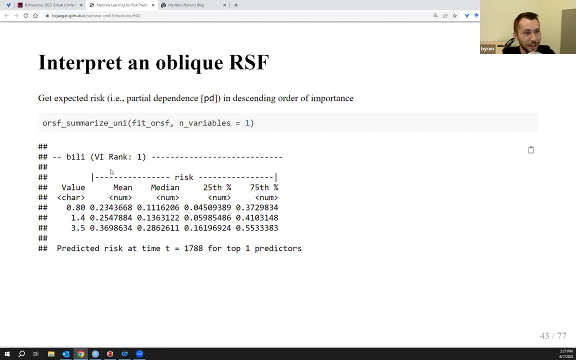 integrate that more into like the main model And that's going to be part of the tidy model as a universe. Alright, so now we can fit an oblique, random survival forest. We'd like to kind of interpret it and get a sense of you know, what are the variables that are important here and how do those variables relate to the predicted risk from the aorsive model? 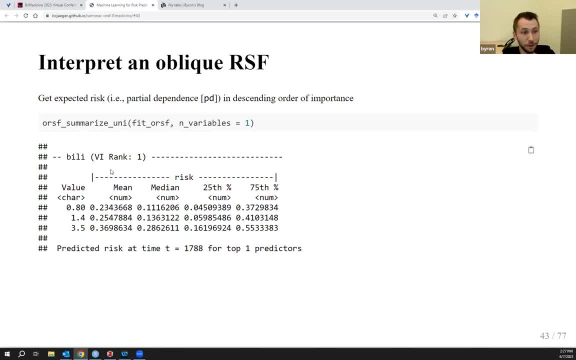 And to kind of give a little bit more background, I just want to touch on this term right here: expected risk. So what I mean by expected risk is: you know, if you have an aorsive model, you're going to be able to do a lot of things. 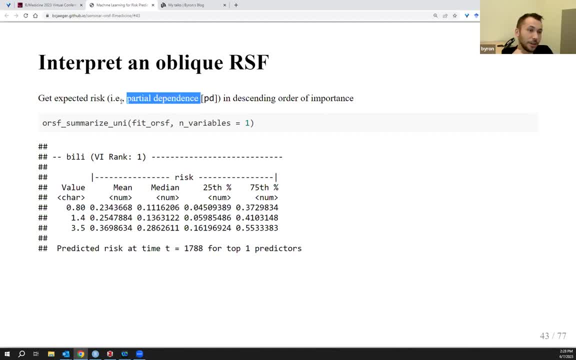 So what I mean by expected risk is actually partial dependence, which is a little bit of a jargon term, But it's a standard thing that people use to look at the behavior of a prediction model, especially if the prediction model is considered black box, like a random forest. 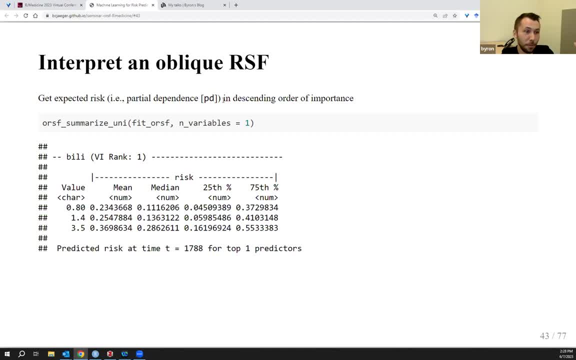 So what it means is we want to understand how a particular predictive variable relates to the predicted risk from a model. So we have a model that uses predictive risk, We have a model that uses this predictor And we want to see how changing that predictor will change the model's expected prediction. 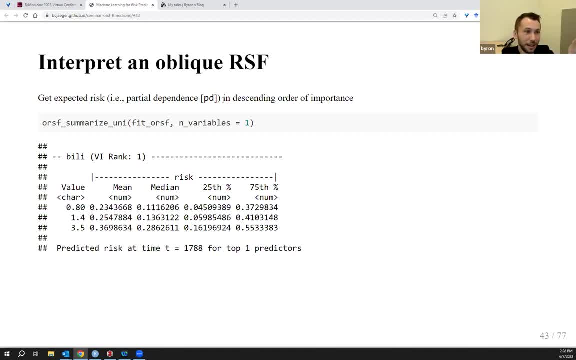 So we kind of set up this procedure where we get our training data and we set every value of our predictor to be a specific value. like we set the value of Billy Rubin to be 0.8.. And then we compute a prediction for all of the observations in our training data, with Billy set at 0.8.. 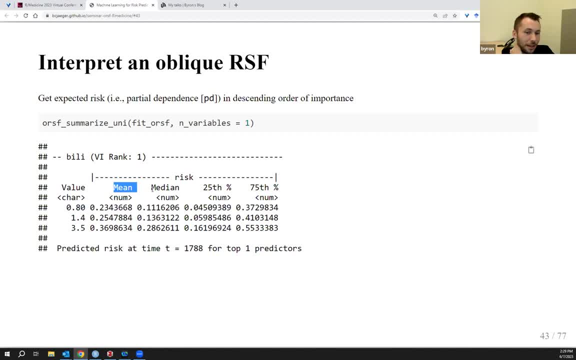 And we take the average of those predictions And we can, you know, take the average by taking the mean or the median or the specific percentile. And then we take the average by taking the mean or the median or the specific percentile. 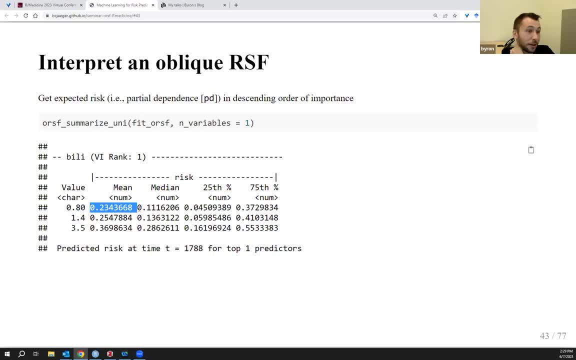 And then we, you know, we present that sum And we do this for several different values of Billy Rubin, to kind of understand what is the expected, predicted risk as Billy Rubin changes and everything else stays the same. So that's actually what ORCIF, Summarize Unity, is going to do for us. 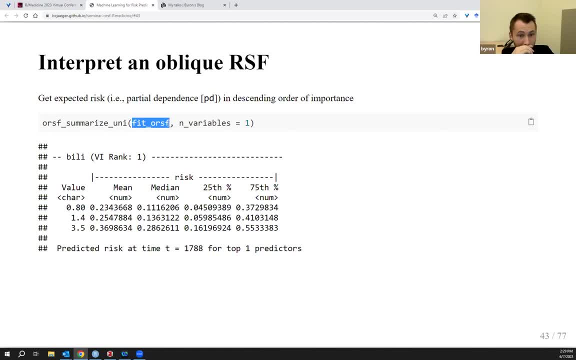 We supply an ORCIF model- That's the first thing we need to give it- And then we tell it how many variables we want to summarize, And then it's going to spit back out a little summary table with a little section for each variable. 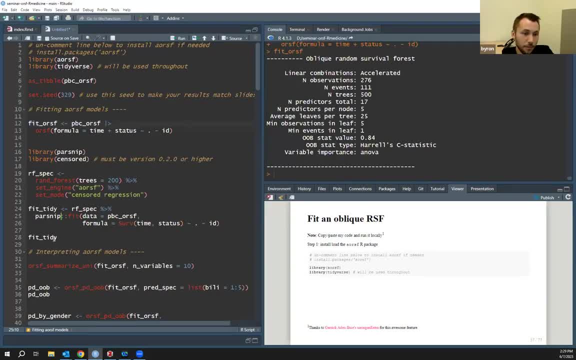 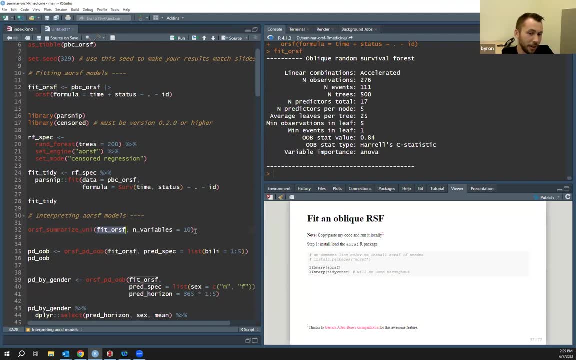 And I'll show you how this looks in our studio session. So here I'm going to run ORCIF Summarize Unity on our fit, But in this notice I'm saying in variables equals 10 here, because I want to actually show you how that looks. 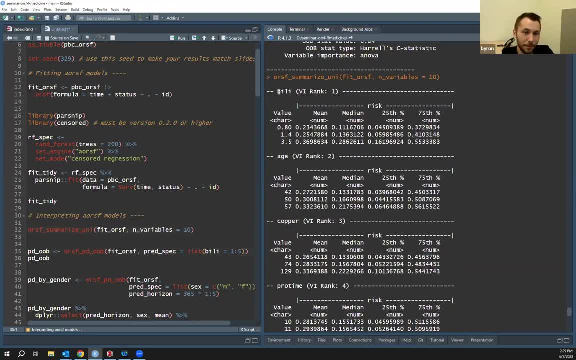 So when I say in variables equals 10, I get back this output where, you know, it's kind of like a table with different sections. It's kind of like a table with different sections. Each predictor variable has its own section And the sections are ordered from the most important variable to the least important variable. 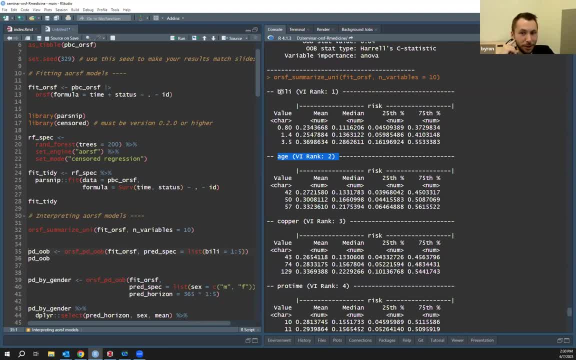 And within each section you can see, you know, for the variable taking a specific value like 0.8, what's the expected risk- Sorry, the expected predicted risk- And what you can do is just look at this little table and get a sense of how the predicted risk changes with respect to that predictor. 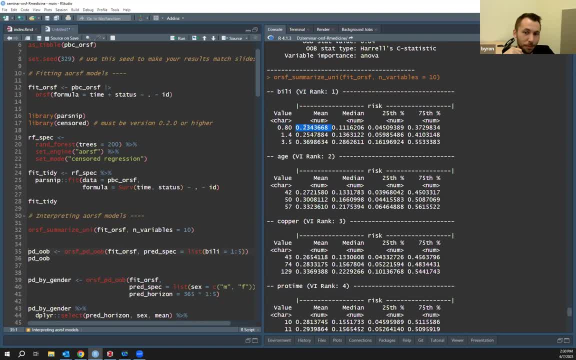 So when Billy is 0.8, the expected, the mean predicted risk is 0.23.. And when Billy is 1.4, the mean predicted risk is 0.25.. A little bit of an increase. you know something to notice. 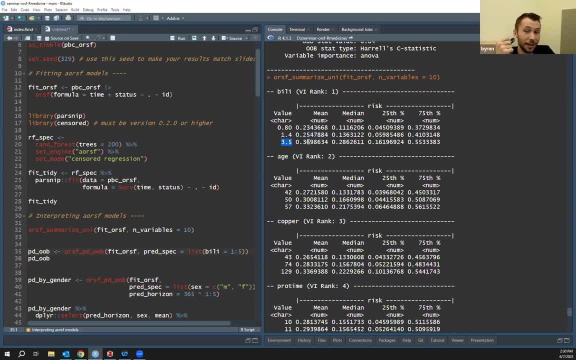 But then when Billy is 3.5, the expected predicted risk is 0.36.. That's a big jump right. So you can understand from that like the expected predicted risk is really increasing a lot when Billy Rubin has gone from 1.4 to 3.5. 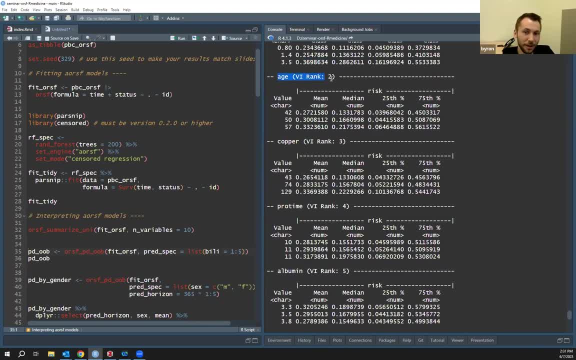 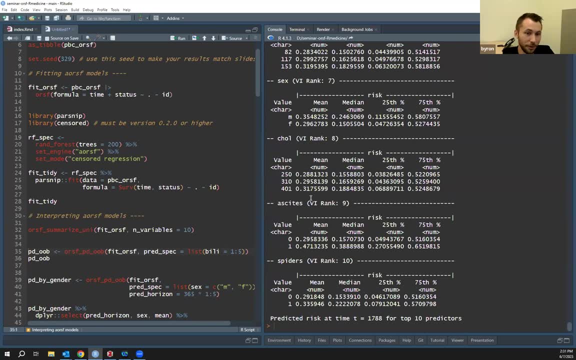 And so you know. you can scroll down through here and see what are the variables that are ranked as important according to this model and get a sense of how the predicted risk changes with respect to those variables. Okay, Back over to the slides. 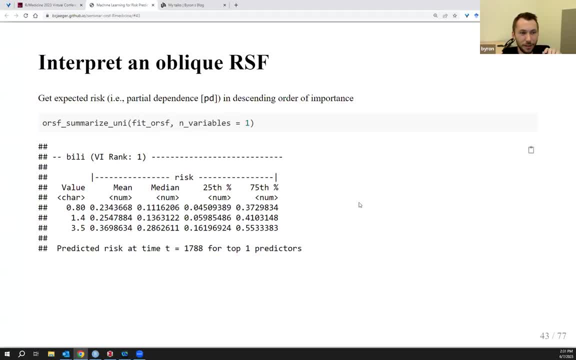 I'll also point out ORCIF Summarize. Uni currently has a bug on some operating systems. So if you do get an error when you run this, it's most likely because of that bug. And long story short, there's a null value in my code. 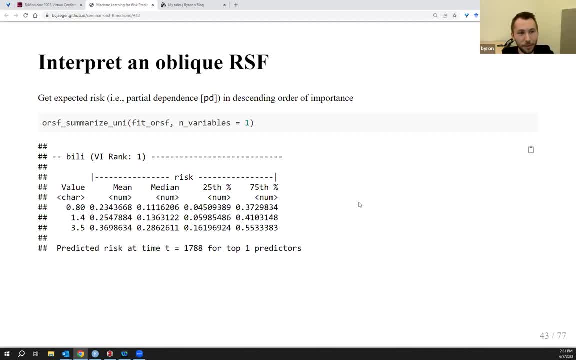 that there should be a false value And I fixed that in the development version. but I didn't want to push that to cram just before this demo because I was worried that I would inadvertently like break the whole package. I know that kind of sounds paranoid. 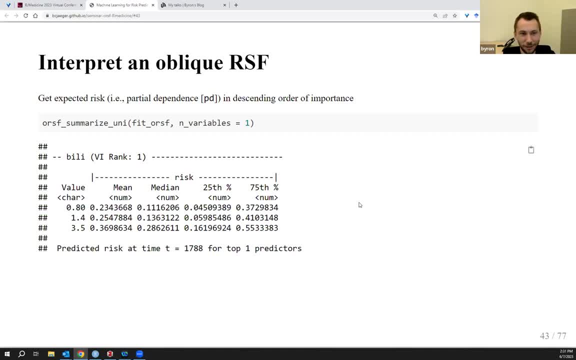 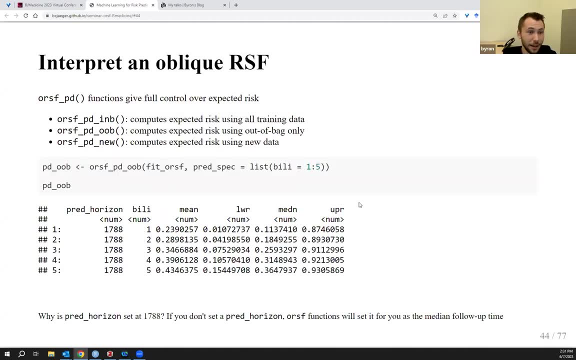 but you know, I thought it'd be safer to just let the bug exist. It's only on some operating systems and it'll be fixed soon enough. So if you get an error with Summarize Uni, no need to worry. 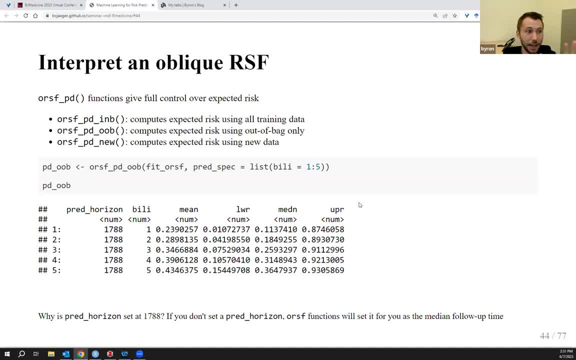 Summarize: Uni is actually based on these functions, which do not have bugs in them as far as I know. These are the partial dependence functions for ORCIF, So ORCIF has these functions to give you a lot more control over how you compute the expected predicted risk. 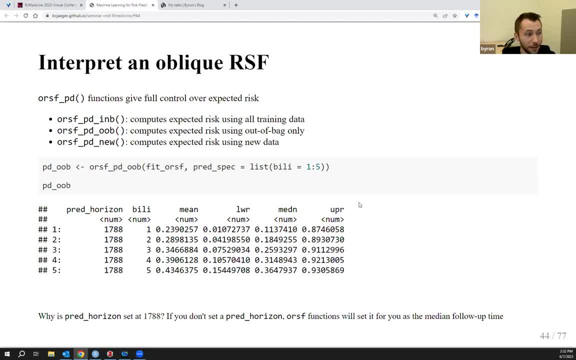 or, you know, partial dependence. There's three different functions that you can access: one that uses in-bag data from the decision trees, another that just uses the out-of-bag data from decision trees, and another that uses data that you would think of as being new to the decision trees. 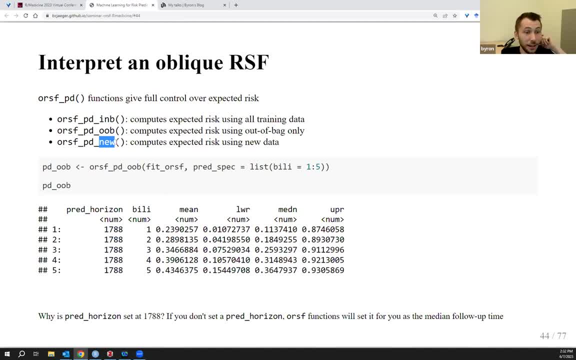 like testing data or your external held-out validation data. So these functions work with two inputs. The first input is going to be an ORCIF model, So I'm just going to supply fit ORCIF to this one. Then the second input is a specification of your predictors. 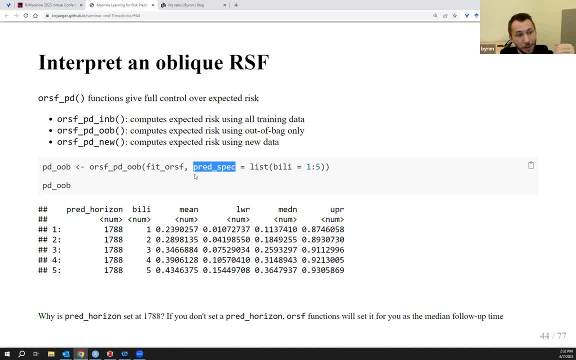 which I abbreviate as predspec. So what you want to do here is supply a named list and the named list will have variables as the names and then the values will be whatever values you want to compute and expect a risk at. So when I say Billy equals 1 through 5,. 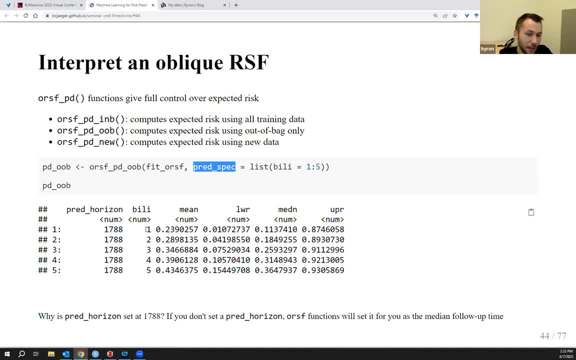 that means that I want to compute expected risk out of the value of Billy equal to 1,, equal to 2,, 3,, 4, and 5.. And so now I get back a very similar table, but I have a lot more control over this table. 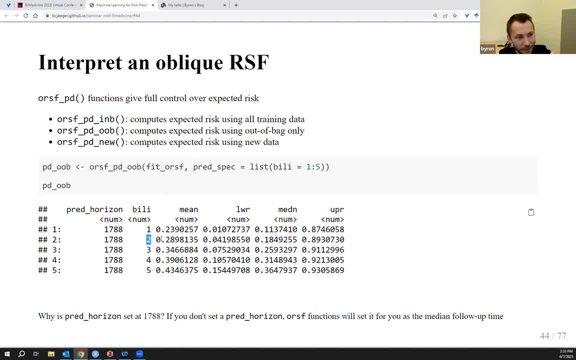 And so now I'm going to talk about this blaring thing that I haven't mentioned yet, which is PredHorizon. You can see that PredHorizon is sitting in this output data set, and each value of PredHorizon is 1788.. 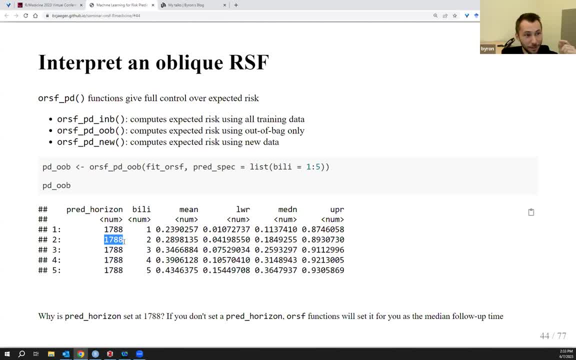 So remember when I mentioned censoring and how we had to directly specify what time we were going to predict the interval to occur over. So we haven't been doing that so far and ORCIF has been noticing that we haven't been specifying any time interval to predict the interval. 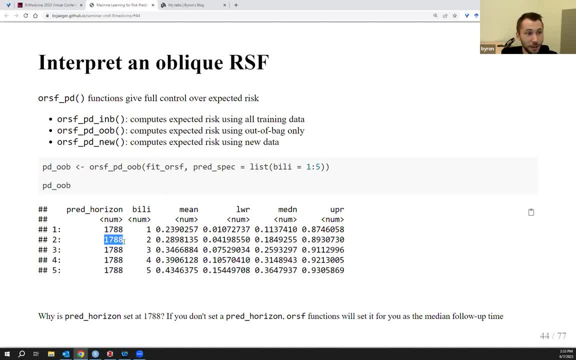 to predict the event's risk over, and so it's kind of just picked one for us. And the way that this works is, if we don't set a prediction horizon, the ORCIF functions will set it for us and they'll just use the median follow-up time. 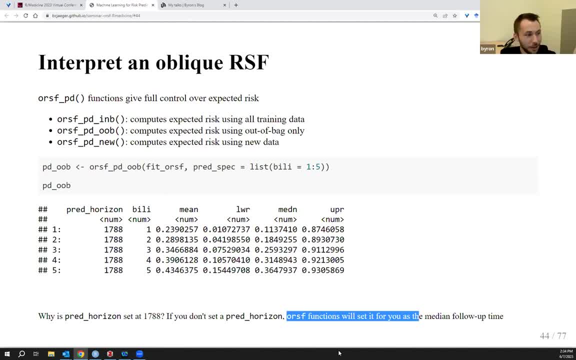 in our training data And I'll just let you in on a secret. Oh, I can recommend a paper for discussing. Oh, sorry, I got distracted by a question in chat. I can definitely recommend a good paper for discussing this partial dependence. 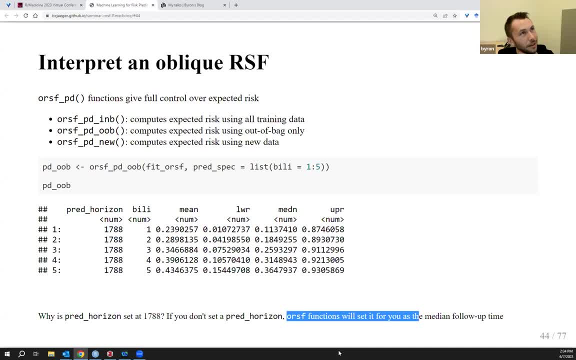 I think the idea was originally brought up in the greedy boosting. I can't remember what it was called. I think it was called reading partitioning algorithm. It was like the original paper for boosting. I'll look for a link for it and try and send it out soon. 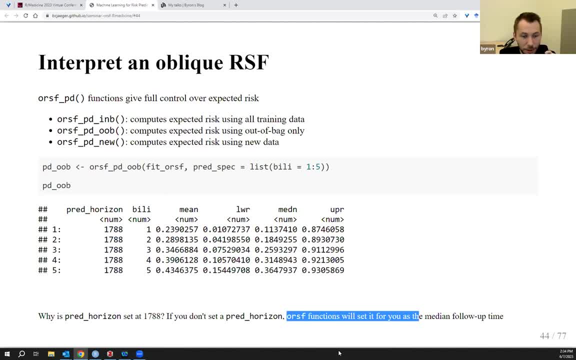 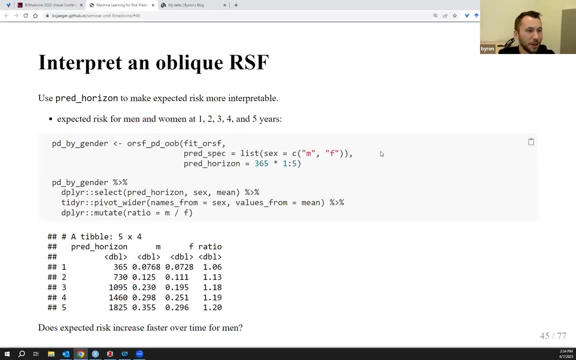 But switching back over to this pred horizon thing, So yeah, so anyway, ORCIF will pick pred horizon for us, and we can sort of- We should actually specify pred horizon ourselves, though, because that'll make our output a lot more interpretable. 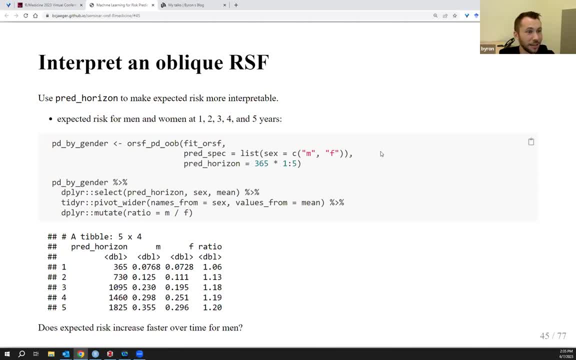 and kind of allow us to put better context around our predictions. So we're going to use pred horizon here to make expected risk more interpretable by saying that we want to predict risk at one year after baseline, two years after baseline, three years, four years. 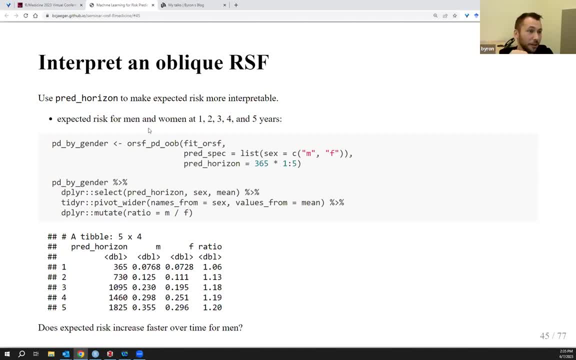 and five years after baseline. And we're also going to expand a little bit on how we're using this partial dependence computer by saying that we want to predict risk for min and min-min separately. So you can see, I've just modified predspec to take sex as the variable. 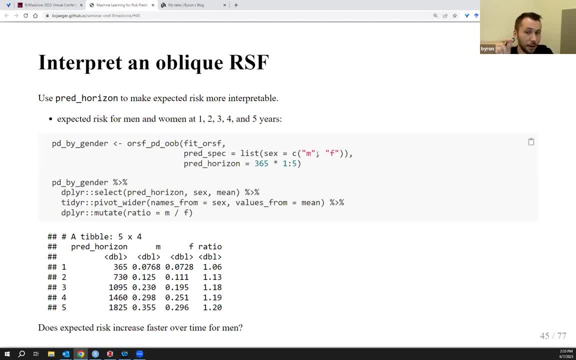 and then computed values of M for male and F for female, And then I'm also going to specify pred horizon. So it's The time scale is in days here. So I'm taking 365 days times the value of one, two, three, four and five. 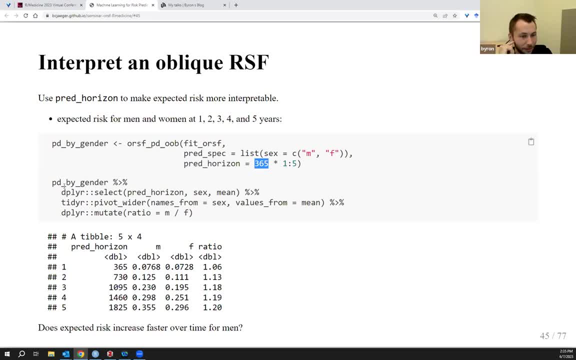 And then, when I get this result back, I'm going to use the tidyverse to put the data into a nice format where it's easy to print out and see all the information. So when you run this, you should get values similar to mine. 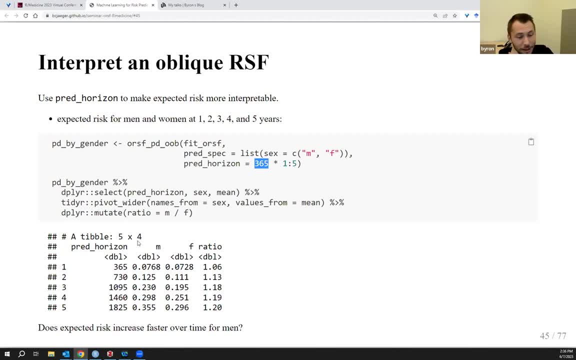 or identical. if you use the same random state as me And you're going to see that the output will show you the prediction horizon of 365,, 730, et cetera, Then it'll show you a column for men and a column for women. 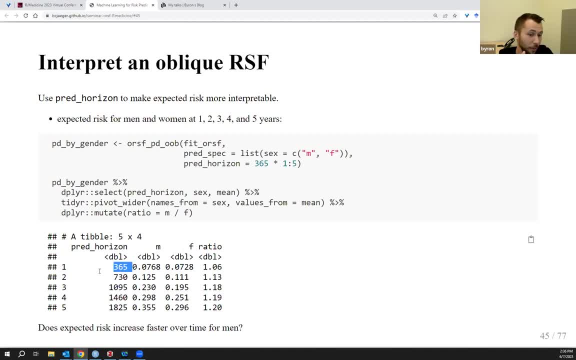 And in these columns you'll be seeing the predicted risk at the corresponding prediction horizon, And I also just added this column here. You can see, I just created a column here called ratio, which is the predicted risk for men divided by the predicted risk for women. 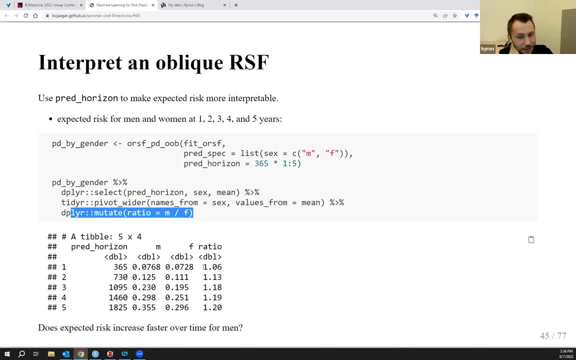 And the reason I added this was because you can see over time that the two groups sort of have a time varying risk, or rather the ratio has a time varying value. The two groups start out at very similar risk, but over time men get slightly higher risk than women. 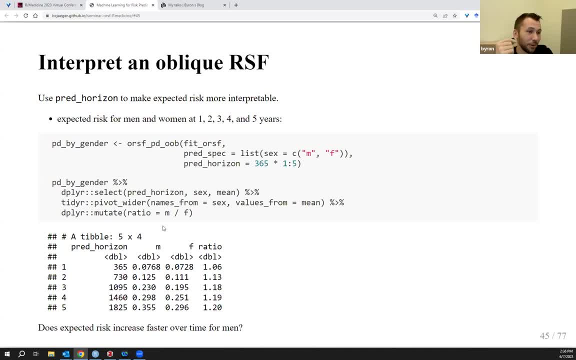 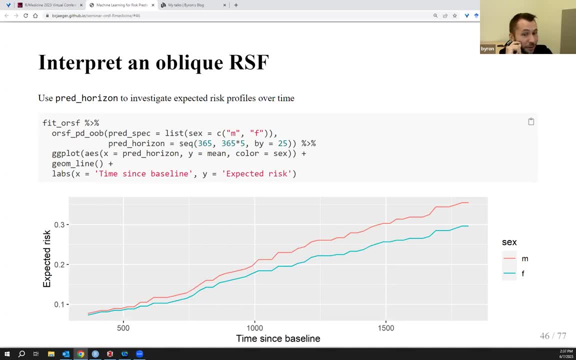 And you can see this also. So you can also kind of bring this out by specifying a finer grid of prediction horizon values, So like, instead of just doing values of one, two, three, four and five years, you can set prediction horizon. 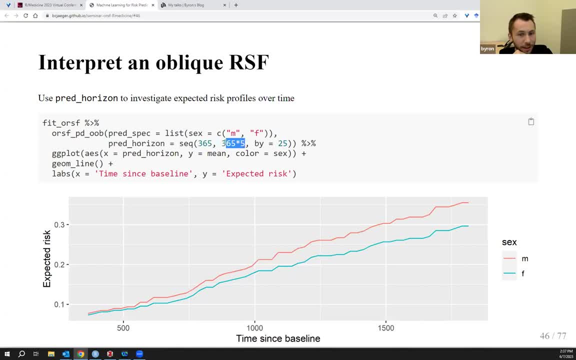 to go from one year up to five years and just take steps of 25 days. So then you get back a data set that you can plot, And I'm using ggplot here, just kind of using the default themes and stuff like that and creating a line plot. 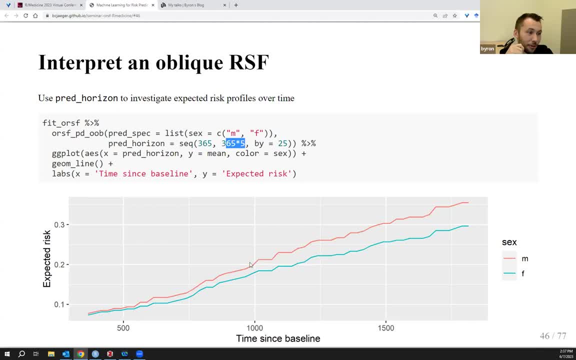 So this line plot is showing us the expected predicted risk for men and women. Men are this line on top, women are on the bottom And it's time since baseline on the x-axis and expected risk on the y-axis And you can see visually. 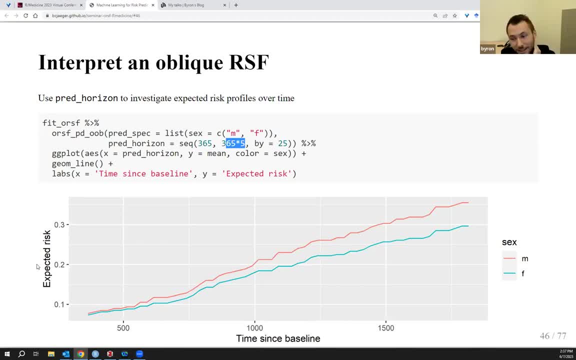 the curves are separating. I tend to think this is a nice thing with oblique range survival forests, because if you were to fit a proportional hazards model, you'll know that proportional hazards models assume that these effects are not time-varying by default. 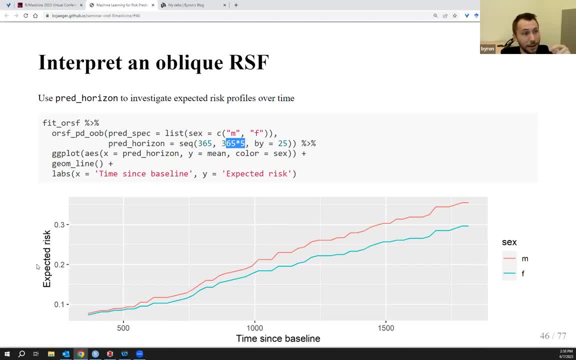 You can set them up so that they do have time-varying effects, but then you'd have to know which effects are time-varying and you may not know that, Whereas with random survival forests, this is done for you and you don't have to know ahead of time. 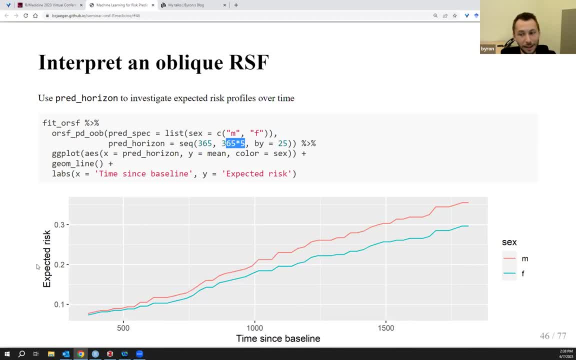 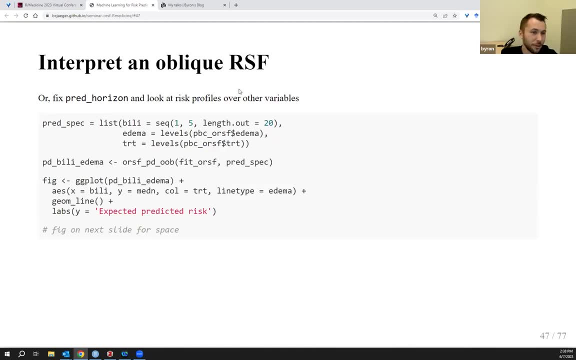 which effects are going to be time-varying and which ones are not. So this is kind of a neat thing with the random survival forest. So now we can also look at this partial dependence output with a fixed prediction horizon, and this allows us to kind of look at 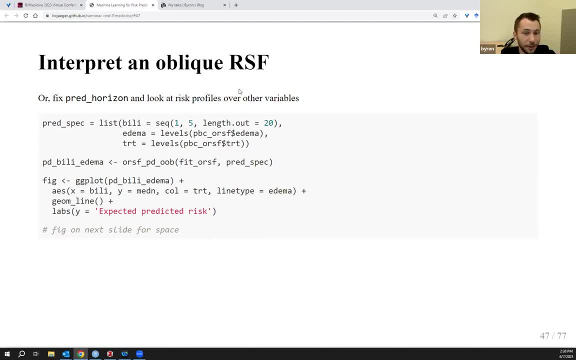 the expected risk profile over multiple variants. So here we're just going to fix the prediction horizon at the medium and we're going to investigate how these three variables may or may not interact with each other. So we've got bilirubin. 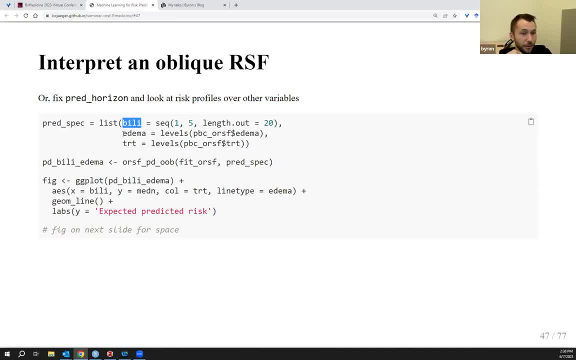 and we've got edema. This is a categorical variable with three levels- and we have treatment, and this is a categorical variable with two levels. And you can see, here I'm kind of just using a shortcut by saying I want to look at edema. 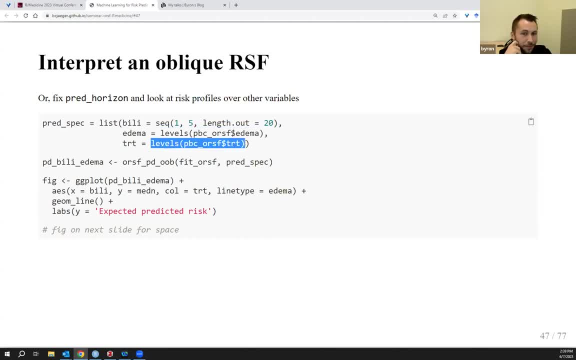 of all of its categories. I'm doing the same thing with treatment and then I'm just setting bilirubin to go from one to five, but I want to have 20 different bilirubin values because I want to look at this in a figure. 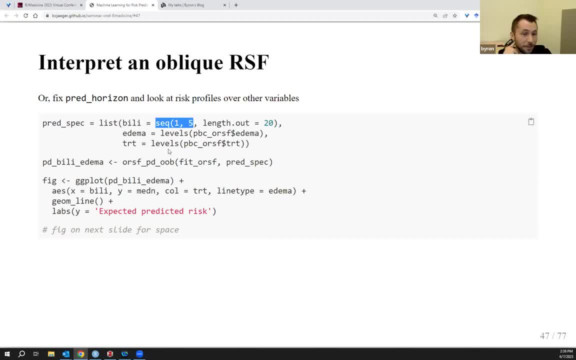 And so now I'm going to run this using this prediction specification, using the same function as before, or this is PD out of bag, and now we're going to get a figure, and I'll probably switch over to RStudio in a second, because I think this is kind of. 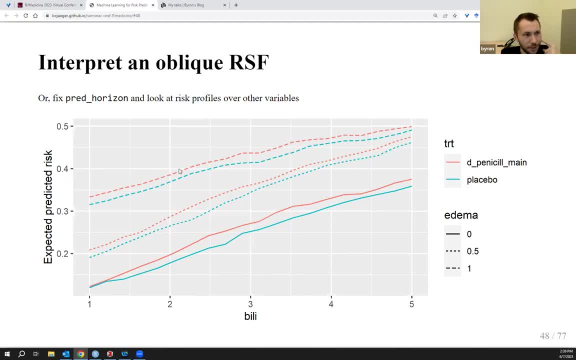 an interesting figure to look at and we can just make sure that the code runs. But when you create this figure, you can see that we have about three different groups here in terms of predicted risk. We've got this group right here, this group in the middle. 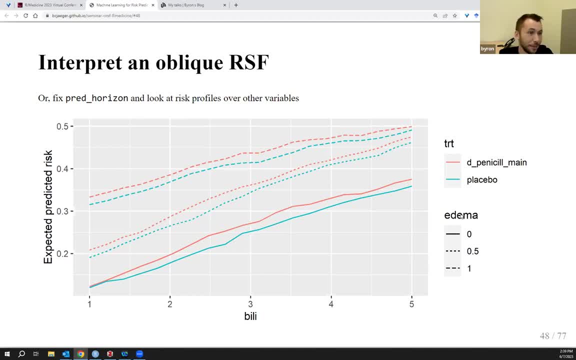 and this group on the bottom. and these groups are really determined by edema status. So edema has a pretty big impact on predicted risk. If it's not, if edema is zero, you're in this group down here. If it's 0.5, you're in the middle. 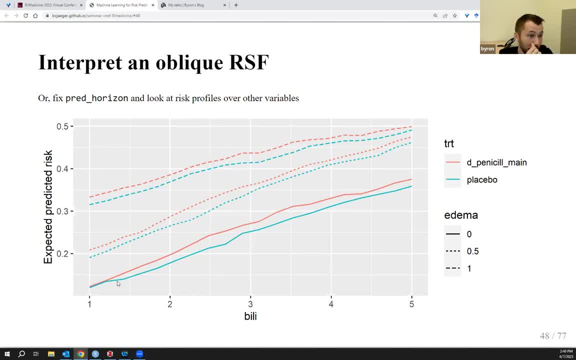 and if it's one, you're up here. But as bilirubin increases, you'll notice that this middle group actually starts out closer to the low-risk group and then, as bilirubin increases, by the time bilirubin is up to five. 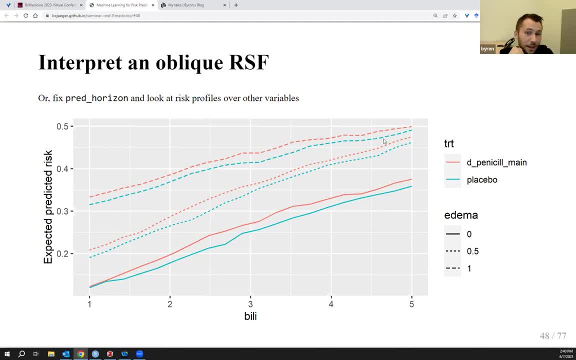 you actually see that this middle group is a lot closer to the high-risk group. So you know, long story short, bilirubin is modifying the relationship between the edema value of 0.5 and predicted risk, And so you could think of this. 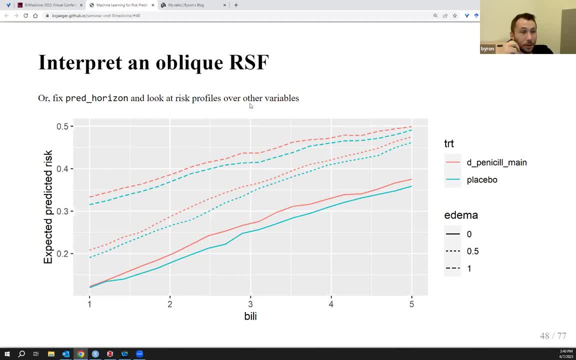 as a two-way variable interaction, and the oblique random survival forest has automatically picked up on this and is showing that to us in this output from the partial dependence function. And so, again, this is nice, because if you're fitting traditional models, you don't necessarily know. 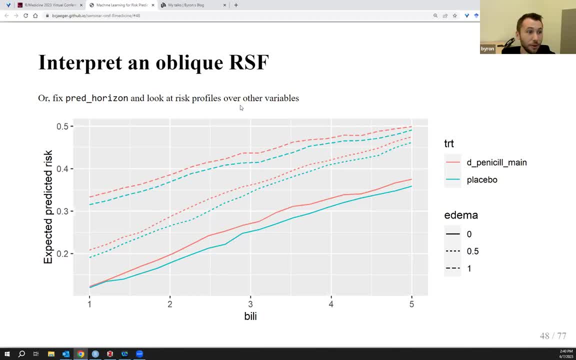 where the two-way interactions exist. but you can fit a random survival forest that'll find them for you and then you can in turn go look for them in the you know interpretation of that random survival forest. So now we're going to pivot. 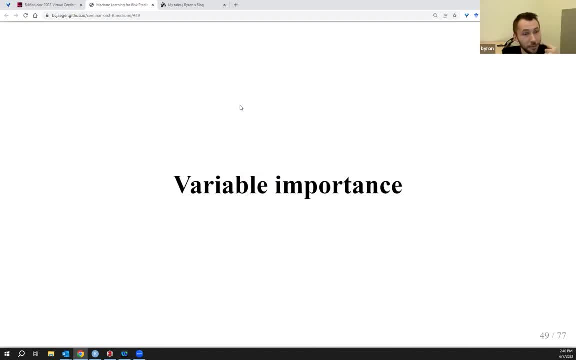 and talk a little bit about another way to interpret the random survival forest, which is variable importance. There are three ways to compute variable importance with the random survival forest in a ORCIF. I'm going to try to cover bare bones of the details. 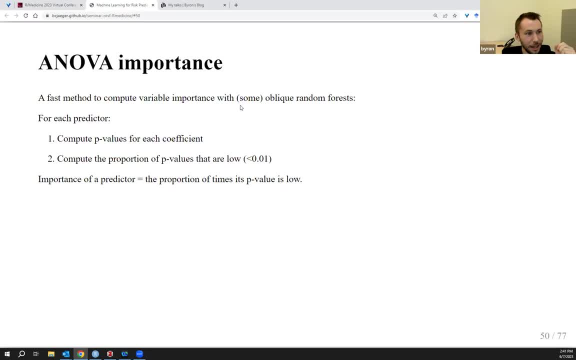 I want to be. I just want to be aware of the time and not spend too much time on the background. So the first way is to compute ANOVA importance, and this comes out of a great paper called called On Oblee Grand Forests. 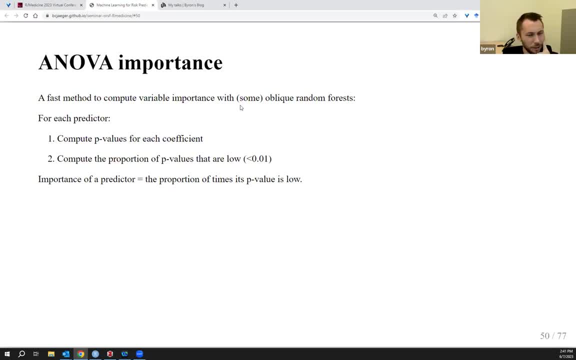 by Menzi. It was published in 2013 or so and there's references for it in the documentation for AORCIF. The basic idea is: when you compute linear combinations of predictors, you're going to find a p-value for each predictor. 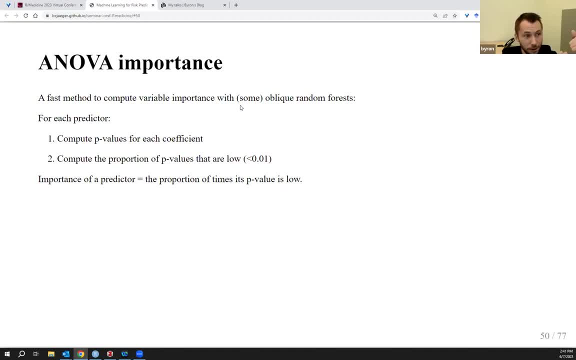 and you'll keep track of the p-values that are corresponding to all the predictors, right? So every predictor has a whole bunch of p-values and you can simply compute the proportion of times that the p-value for a predictor was very low and that proportion is going to be. 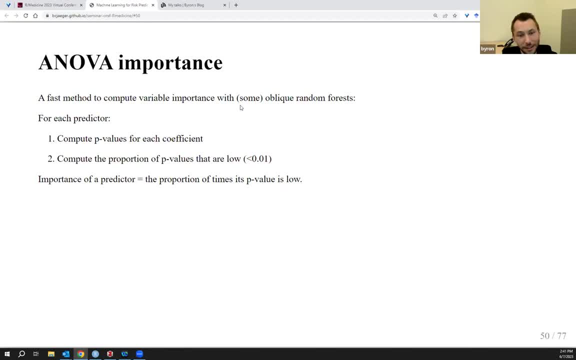 the importance of the predictor. So the idea is, if the predictor always has a very low p-value, it's probably important, And if it's always got a not so low p-value, then it probably isn't that important. And so obviously this is like: 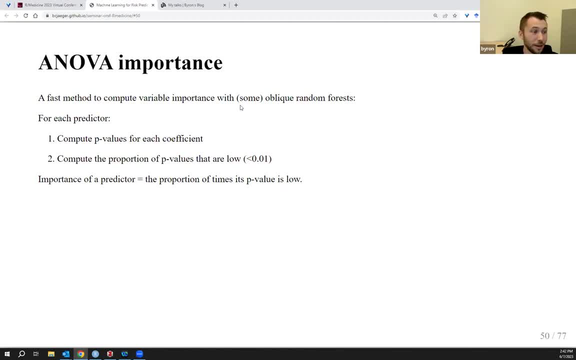 going to have some limitations, but it's one thing that's great about it is it's very fast. Another way to compute variable importance is this more traditional method of permutation. This is where you've got a forest that you've already fitted and you know it's prediction error. 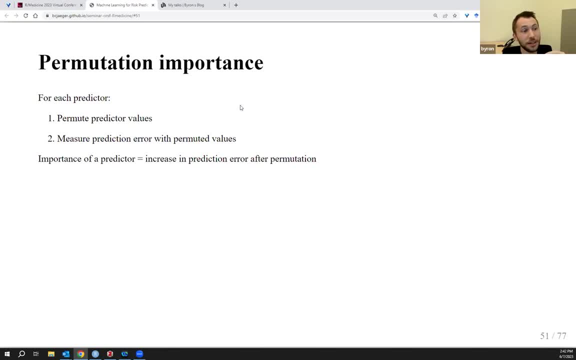 So now you're going to permute a predictor and then you're going to reassess what the prediction error is after the predictor has been permuted. So what that looks like is we have a fitted forest here and I'm going to permute. 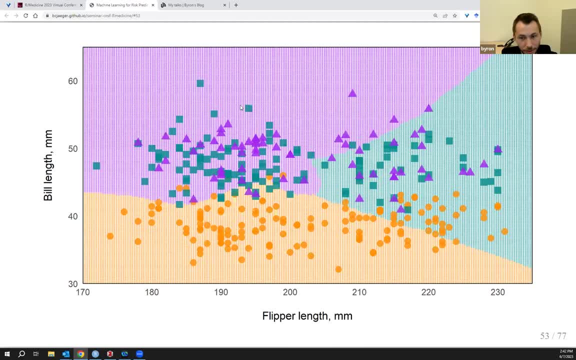 the value of flipper length. So here we go. Oh, it's been permuted And now we can see from the picture that we actually have a lot of misclassified points, All these you know gentoo penguins that were originally classified. 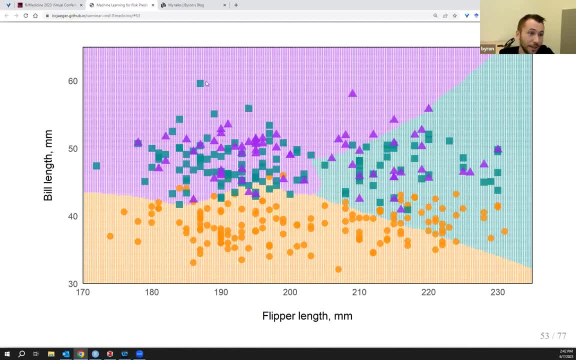 as gentoo's are now being classified as chinstraps and that's incorrect. So we can see that permuting this variable has really messed up our random forest prediction accuracy and we can quantify how important that variable is by how much worse. 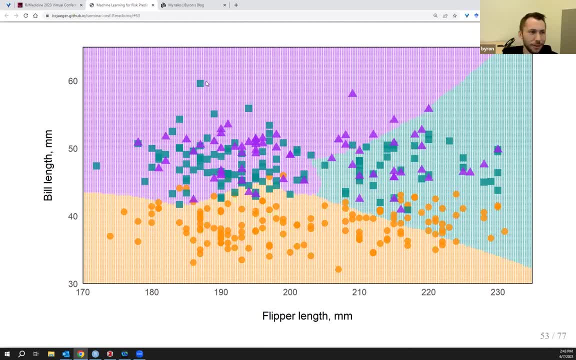 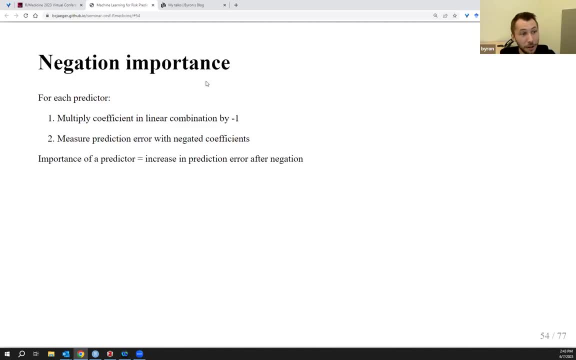 the prediction accuracy got. So- and this is kind of- I'm a little hand-wavy here- This isn't exactly how it works with the picture, but it's the concept. So another way to compute variable importance with aorsif is to use something called. 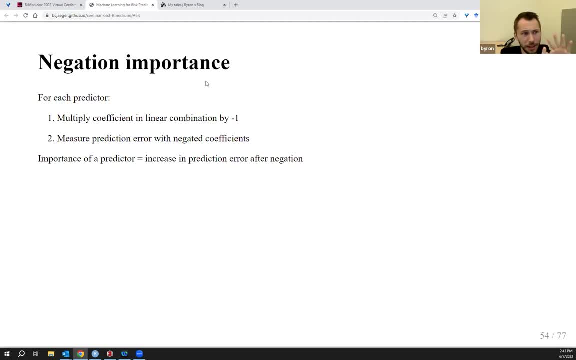 negation importance. and this is similar to permutation, but it has a little bit of a different velocity. So actually, for each predictor, instead of permuting the values, we're going to go into the forest itself and multiply that predictor's coefficients by negative one. 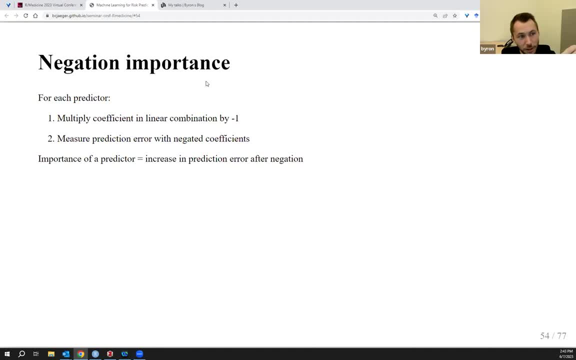 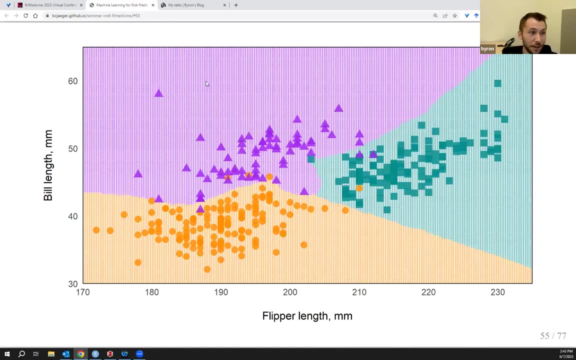 So if it's in a combination of predictors that its coefficient is like 1.6 or something, then that's going to be converted over to negative 1.6. And what this effectively does is it removes the slope of the decision boundaries in the trees. 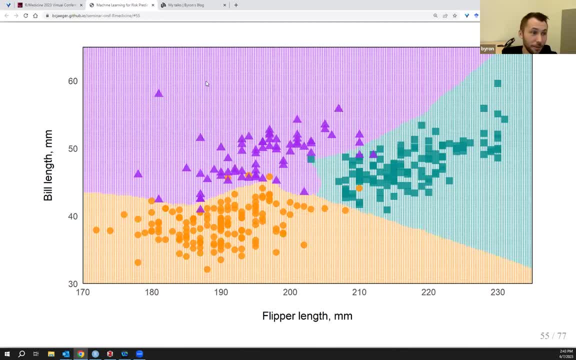 So again a little hand-waving here, but what this conceptually means is that we have a fitted forest here and instead of permuting the values, we're actually going to flip the decision boundary. And when we do this, we can see that we again. 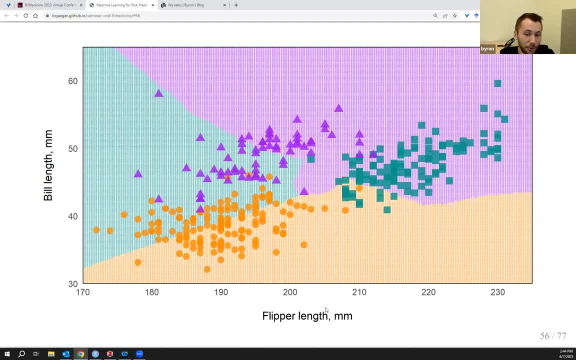 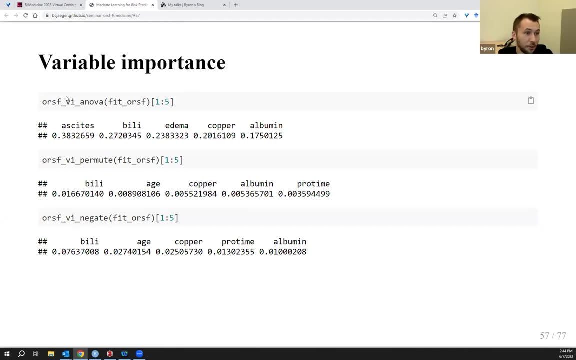 have a lot of misclassified points And because we flipped all the decision boundaries just based off of flipper length, we can conclude that flipper length is an important variable. So all three of these methods are accessible in a ORCIF. There's sort of a family of functions. 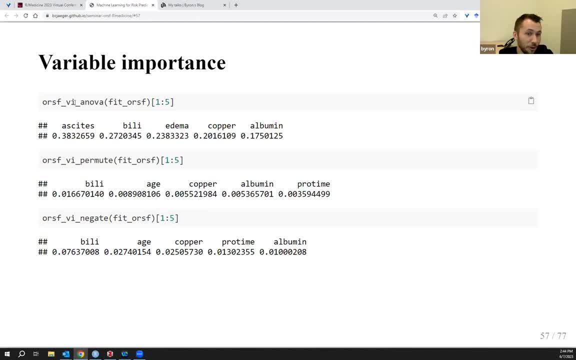 called ORCIF underscore VI for variable importance, And you can run that function on a fitted ORCIF model, like I'm doing here, And you can also just specify when you fit the ORCIF model what type of importance you want to compute. 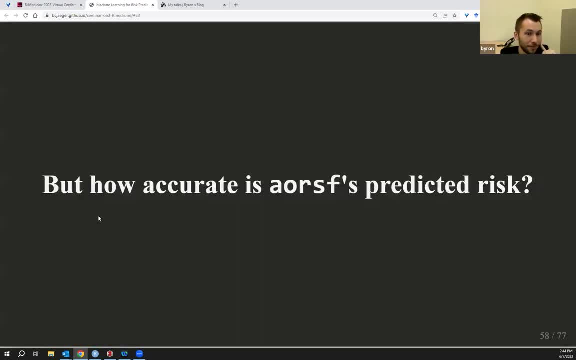 All right, So there's two ways of getting about it. Okay. So we're now at the point where we can ask a question. You know, we see that we can fit these ORCIF models and we can interpret them, but it's kind of important. 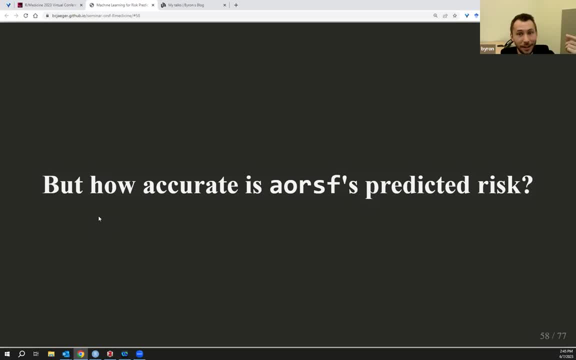 that they give us predicted risk. that is somewhat accurate because there's not much point to interpreting predicted risk if the predicted risk isn't, you know, a good predictor of what's actually going to happen. So I've run a larger benchmark in my preprint on archives. 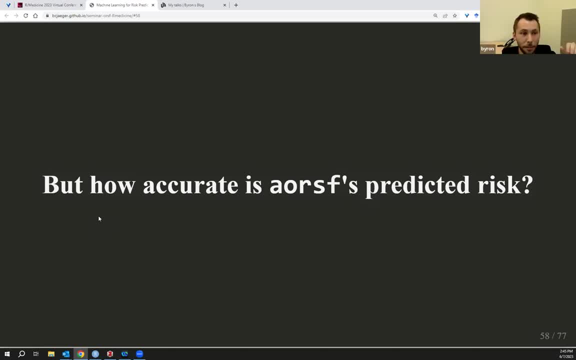 over 35 different prediction tasks. But in the demo here we're going to look at a smaller benchmark over about 11 different prediction tasks, And you will be able to run this on your own systems if you want. But just a fair word of warning. 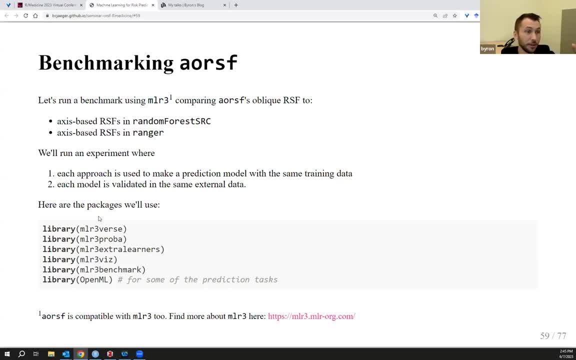 you'll have to install MLR3 and the associated R packages for survival with MLR3. And some of these are not on CRAN, So it'll just take a little bit of extra legwork to get them up and running on your system. 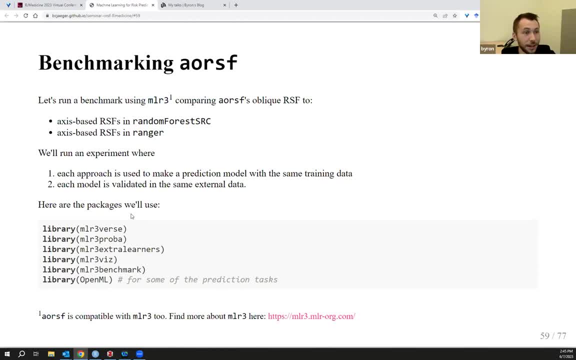 Luckily, you can also just follow along with the slides and take my word for it that I'm not making up the results, which I'm not. So what you'll see here is all the packages that I need to load from this benchmark And what you'll see up here. 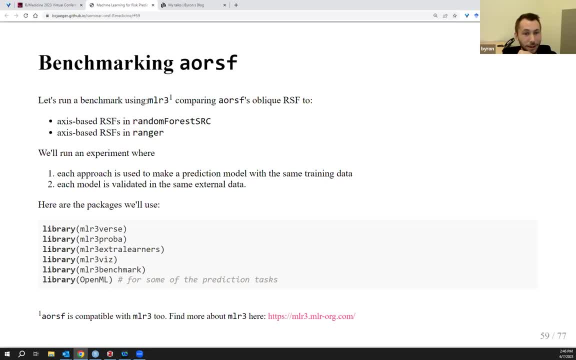 is kind of what the benchmark is going to do. We're going to use MLR3 and we're going to be comparing the prediction accuracy of models with a ORCIF to the prediction accuracy of some random survival forests that use axis-based trees. 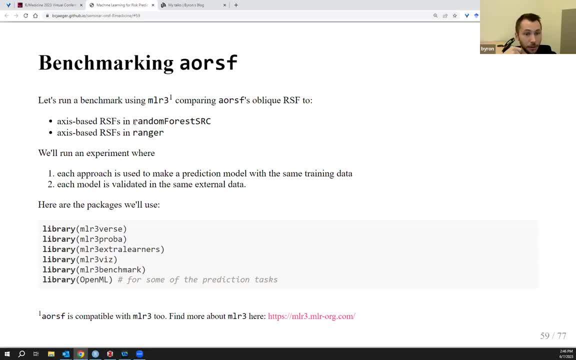 In particular, we're going to be using the random forest SRC package, which does survival, regression and classification forests, And then we're also going to be using axis-based random survival forests from Ranger. So you may have used these packages before and you may not have. 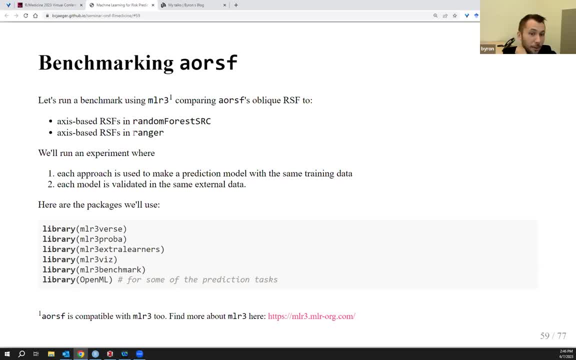 but the general idea is that these are very widely used R packages for random forests and they're quite good, very good, random forest packages. So we're going to run this experiment where we basically fit the model with each of these three different learners. 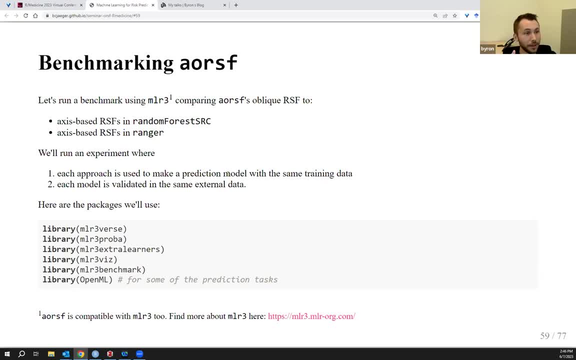 And then we validate that model in some held out testing data And now I'm just going to flip through some slides to show you where I'm getting that testing data or that data from. So first we'll use our PDC ORCIF data. 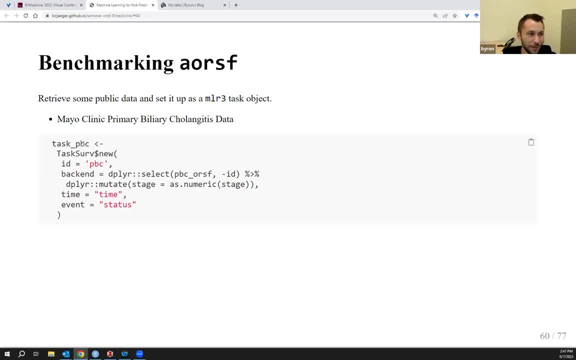 And you can see that I'm making this thing called the task. That's because the general syntax of MLR3 is one where you create tasks for prediction, So that's why I'm using this task name. I've got another task with data. 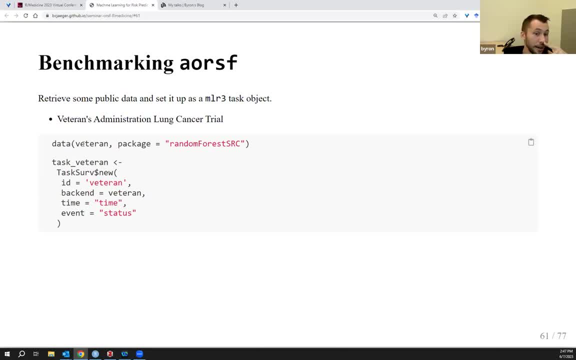 from the Veterans Administration 1 cancer trial, And this data actually comes directly from random forest SRC, so it's pretty easy to make a task with it. Some other data that I'm pulling out of the OpenML R library. OpenML is a very handy R package. 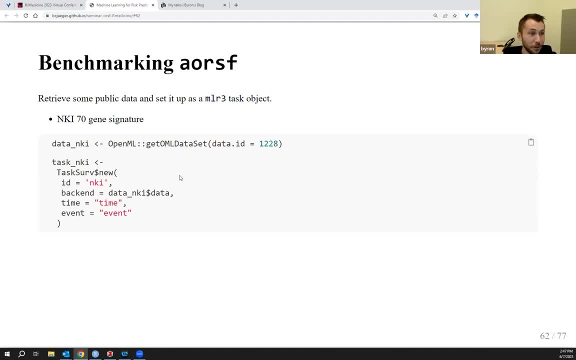 You can just grab data sets that are publicly available and download them from the OpenML website. Another data set from OpenML: lung cancer. Another data set, this one's coming out of I'm not quite sure, oh, out of the survival package. 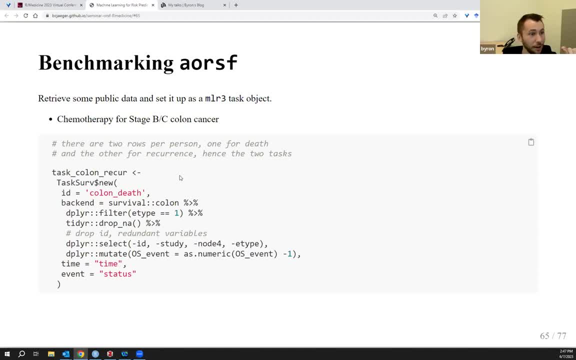 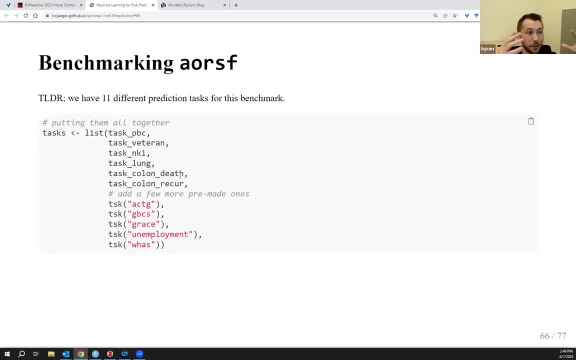 And this is from a cancer trial. This cancer trial actually had two survival outcomes, And so we're making a separate prediction task for each of those two outcomes. And now we're going to put all the tasks together in a list And you can see at the bottom of the list. 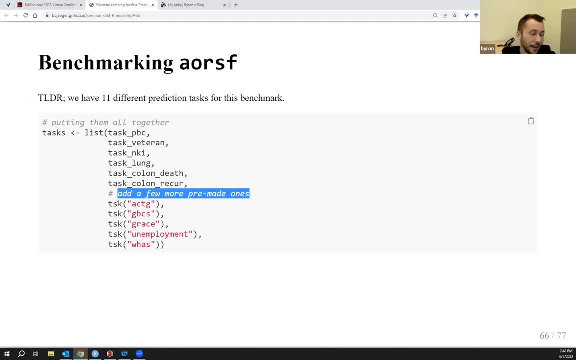 there's a couple more pre-made tasks, And these are just tasks that are already available with MMR3.. So we've got 11 different prediction tasks in total And we're going to set up a little benchmark where we go through each task separately. 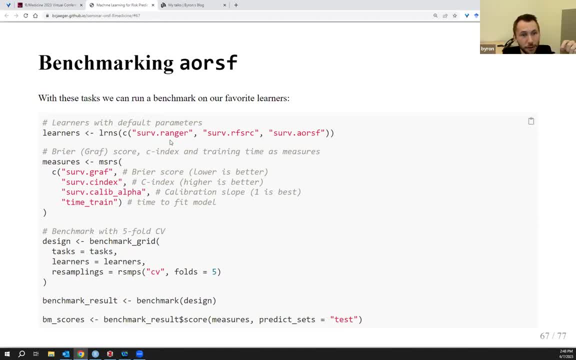 And with each task we're going to be running five-fold cross-validation. So we start with the full data, split the data up into a training set and a testing set. On the training set we'll fit three models: one with ORCIF. 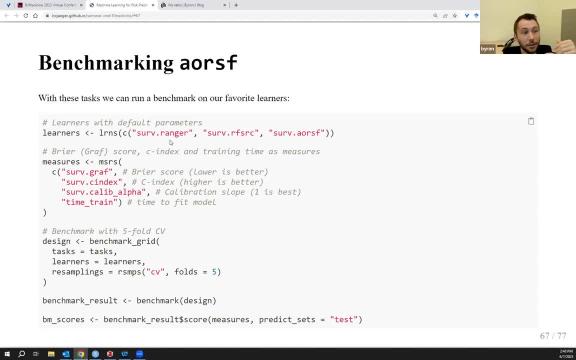 one with random forest SRC, one with Ranger, And then each of these models will make predictions for the testing set, And we'll evaluate how accurate those predictions are. And so here we're saying: these are the learners that we want to use. 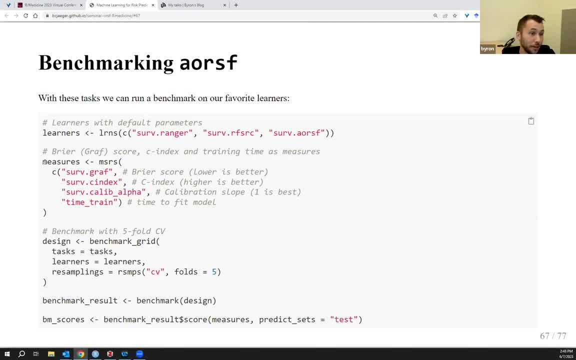 And then we're going to say: here's how we want to evaluate the accuracy of those learners. We'll give a graph score, which is also a Breyer score. I hope you've heard of at least one of those. I don't have enough time. 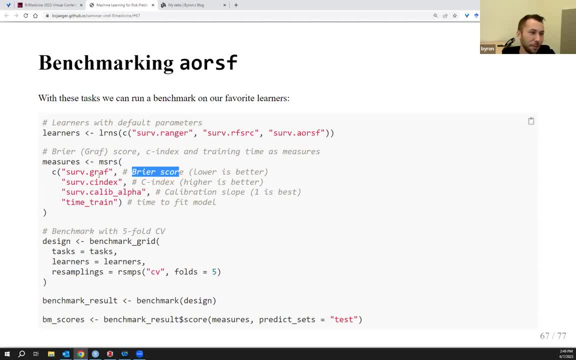 to really go into what they mean, but I'll just say: lower values are better for the graph score. We're computing a C index which is going to tell us how well a model discriminates between cases and non-cases. We're going to compute a calibration score. 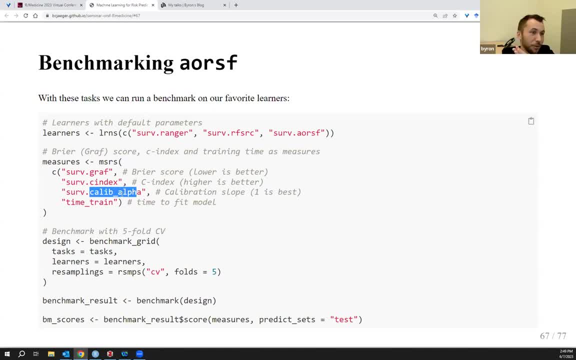 And so this is a slope that we want to be equal to exactly one. The closer to one it is the better. And then we're also going to keep track of how long it takes to train our models, because, as I mentioned before, 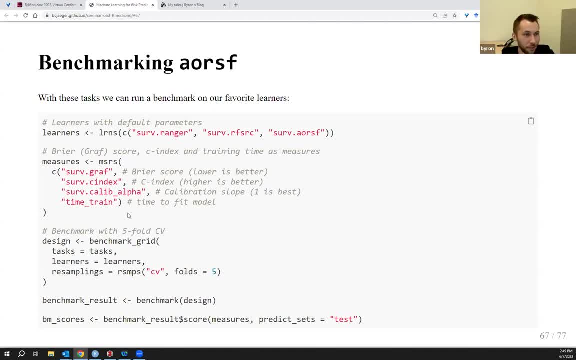 people prefer not to use slow software, So faster software is nice, assuming it works. And then we actually create our benchmark. That's what this code is going to do, And then we'll run the benchmark and we'll pull out the scores of these three different models. 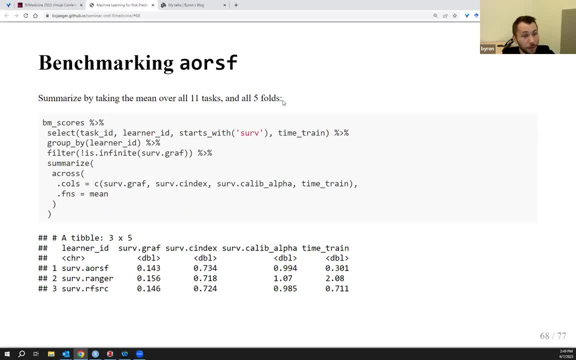 So when we do this we can summarize the results with this bit of code here. You can see this is just kind of a little bit of tidyverse mixed in with. Well, this is basically just tidyverse stuff, And here's the summary. 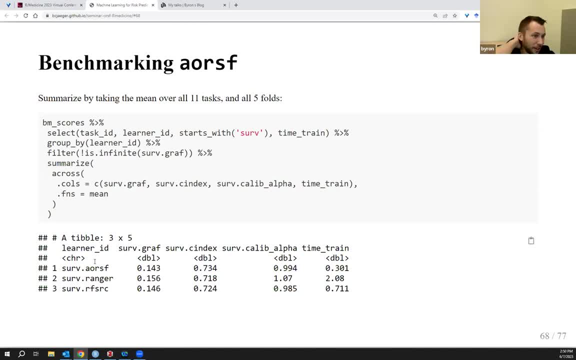 All right. so this is where we're actually able to compare the prediction performance of our different learners here. So the graph score column- we can see the expected graph score over all 11 prediction tasks And the average for AORCIF is 0.143.. 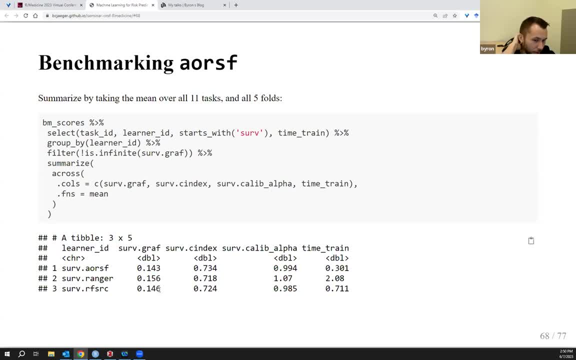 And then the average over here is 0.146 for Random Forest SRC and 0.156 for Ranger. So remember the graph: score lower is better, And so AORCIF kind of gets a little bit better score here. The C index. 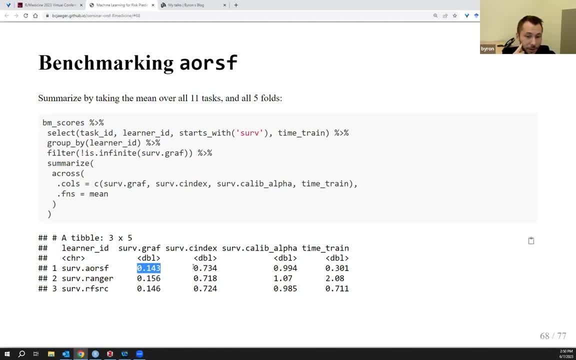 now it's higher- is better than the C index. So AORCIF gets a score of 0.734.. Random Forest SRC is just a little bit below that, And then Ranger is just a little bit below that. Next up is the calibration. 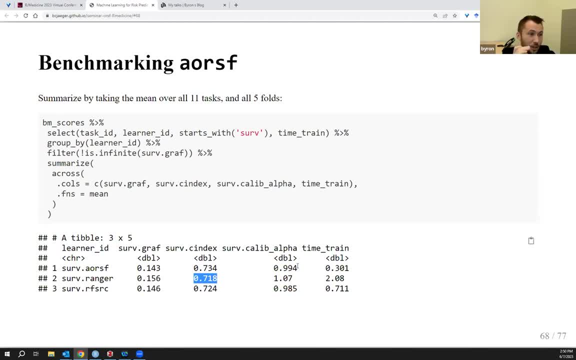 The closer to one the better. So a perfect calibration gets a value of one for the calibration slope, And AORCIF is coming in at 0.994.. Random Forest SRC comes in at 0.985, a little bit further away from one. 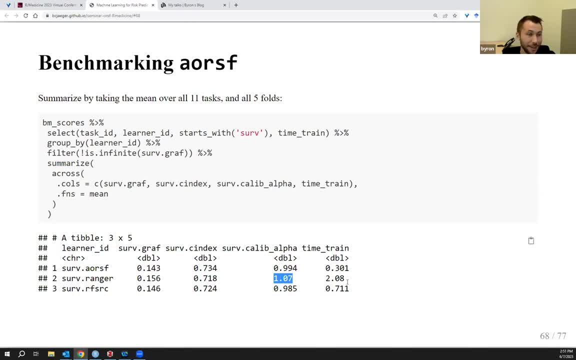 And then Ranger comes in at 1.07.. And then, very last thing, I realize I'm just reading a table to you, but all this is valuable information, So I'm just going to kind of cover it. Next last thing is the time to train. 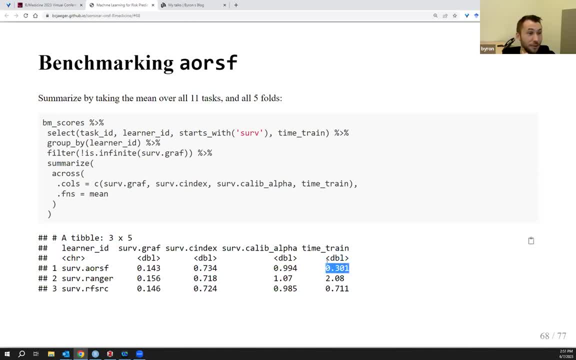 So here you can actually see AORCIF is efficient, which is great, because oblique trees are actually very hard to fit efficiently, And that's been the main challenge of developing AORCIF. It's like: how do I fit these trees? 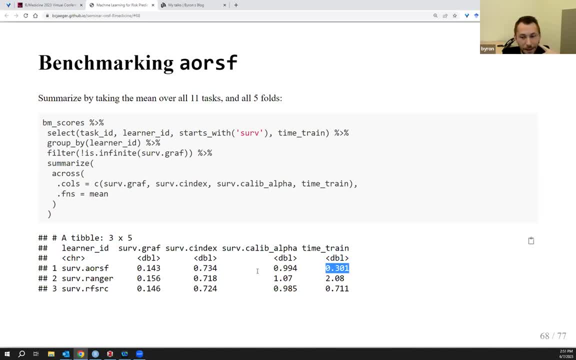 in a way that won't take days to finish And if you're interested in exactly how AORCIF actually does do this quickly. the archive preprint has quite a lot of details on that. I'm not going to go into it here. 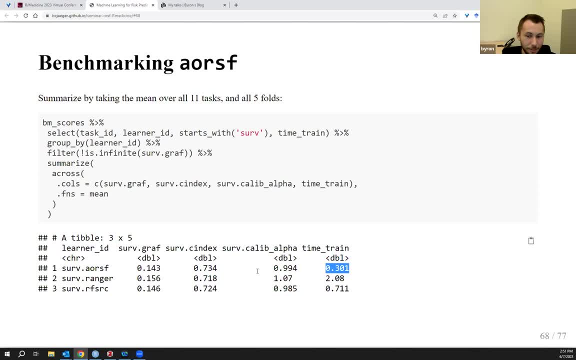 because this is just demonstrating AORCIF and how to use it, But I find it interesting. I will say the caveat here is that MLR3 has forced these learners to run on a single processor, And Ranger and RFSRC are both designed. 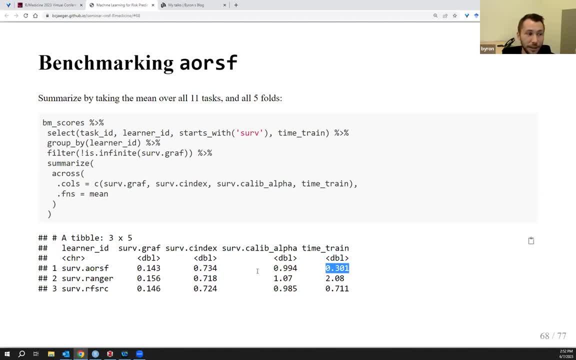 to be run in parallel. AORCIF is not quite. Oh, good question about the scale. That's in seconds, I believe. So on average that's the number of seconds it took to fit a model. Thank you for that question. 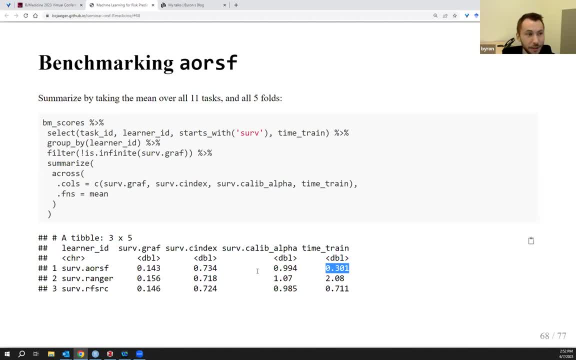 It's a very good question And so the comparison here is a little bit biased because AORCIF never even I didn't write AORCIF to use parallel processing. I probably will at some point. But Ranger and RFSRC expect to do parallel processing. 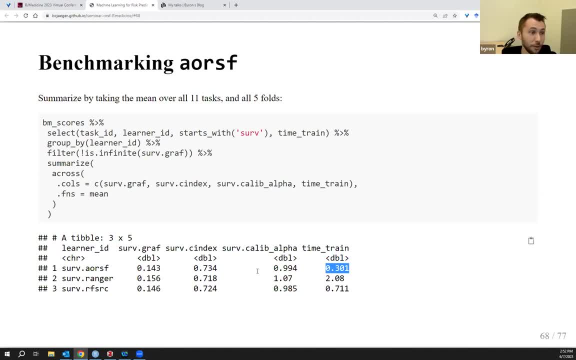 And when they do, they run very efficiently, more efficiently than AORCIF in many ways. So it's a little bit biased. I wouldn't take this as a final say on the efficiency of these R packages, but it does at least show that AORCIF is not slow. 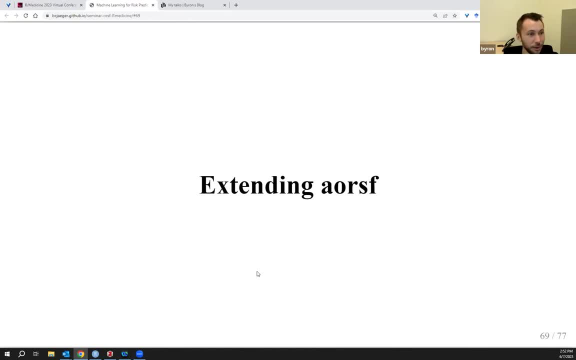 So now we'll just briefly touch on how you can take AORCIF and tailor it a little bit so that if you don't like the prebuilt way that AORCIF finds linear combinations of predictor variables, you have a lot of control of that. 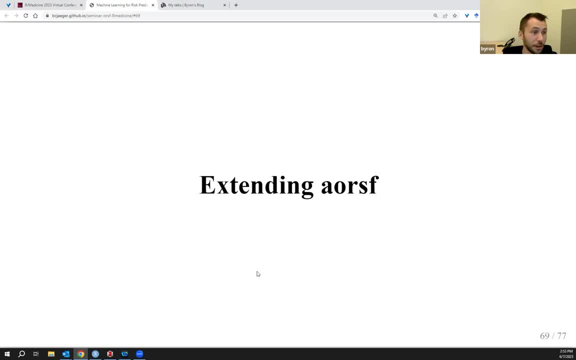 You can change that and modify it to do exactly what you want it to do. So when you fit AORCIF models, you can supply this control argument, And the control argument should be the output of one of these different control functions, And there's four functions available right now. 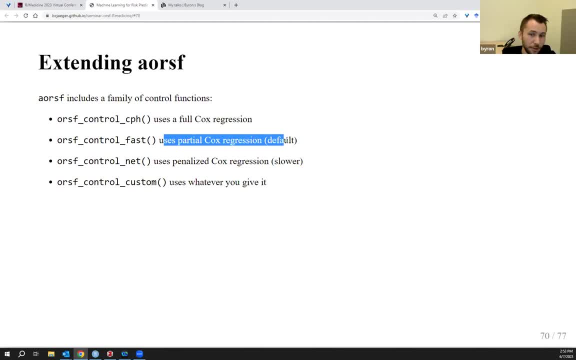 The default one is to do the fast version of AORCIF, So this just runs the fastest. And then you can also use: instead of fitting this like partial Cox regression model, you can fit a penalized Cox regression model which runs substantially slower. 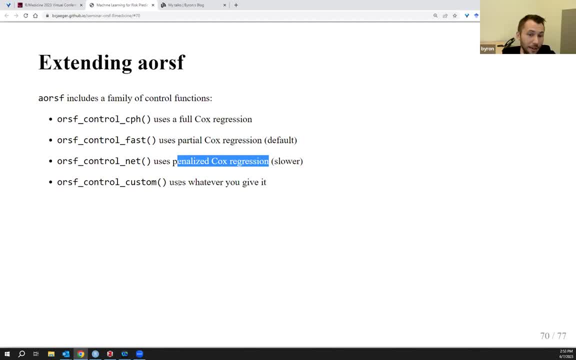 but it does perform better in some cases. And the one that I find the most interesting is the control custom function, And I'll show you how to use this in a second. but this allows you to create your own function for finding linear combination of predictors. 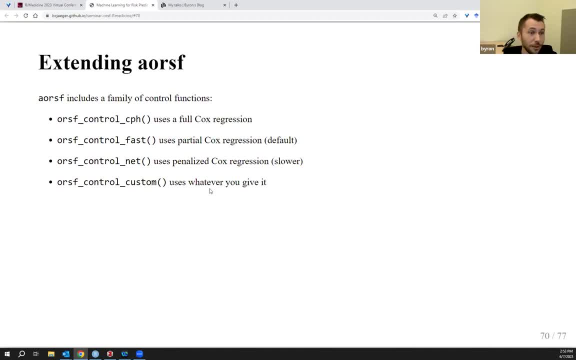 And then you just supply that function to AORCIF and it takes it and uses it for you. So here's how that works. Let's say that I wanted to make an oblique, random survival forest And instead of finding this linear combination, 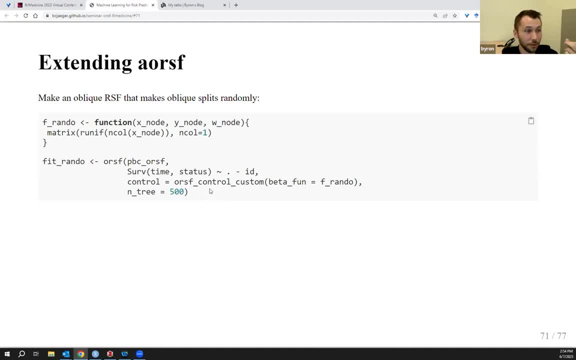 predictors with Cox regression. I just want to find some random coefficients and combine my variables that way. So I'm going to make a function called F underscore random for making random linear combinations. And all this function does is it returns a matrix of values from a random uniform distribution. 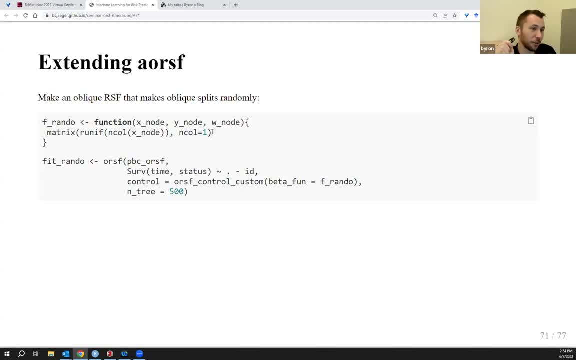 And then that matrix will be used as my linear, the coefficients for my linear combination. So then I take this function and I pass it into the AORCIF control custom function, which then I pass into the control argument of AORCIF. 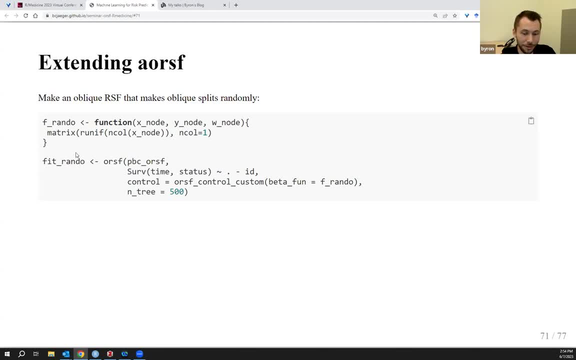 And now I get back my customized oblique, random survival forest, And there's a lot of different things you can try with this. Maybe you don't want to do random coefficients, Maybe you actually want to apply principal component analysis and use that as a way to find a linear combination of predictors. 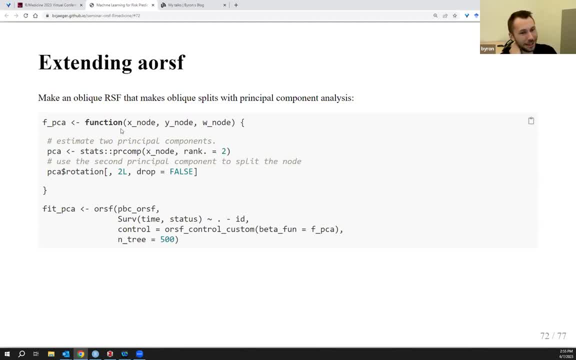 And so I'm not the biggest expert in principal component analysis, but I can at least write a function that uses the PR comp function and then pull out one of the principal components from that. And here I'm actually pulling out the second one, because when I experimented with this 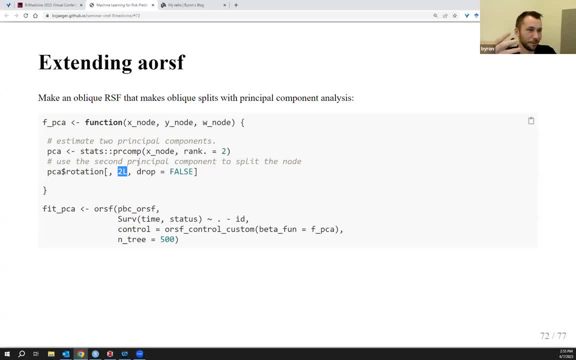 the first one was more or less dominated by one variable, So it's like that's basically just fitting an axis based forest. But the second dimension was more good mix of variables. So that's why I'm using the second dimension, But then I just pass this in. 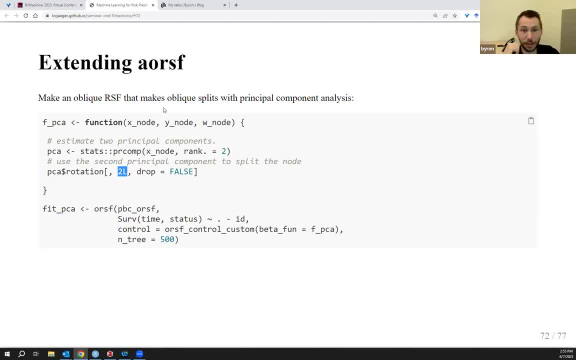 and now I'm using the principal component, analysis, to fit an oblique random survival forest, And so you can write these functions yourself and you have a good bit of control over how the random survival forest works. And, of course, the thing that I'm not really mentioning is 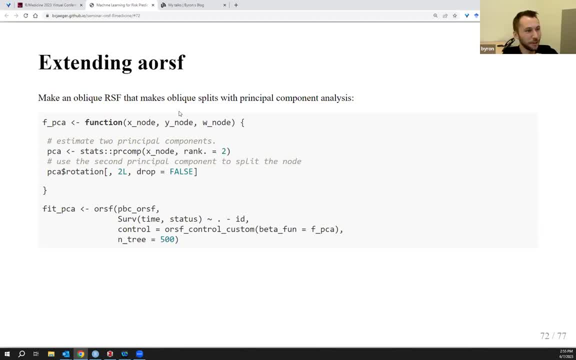 it's very easy to cause your R session to crash if you send R functions into C++. So when you do this, there are some nice error. There are some functions within AORCIF that'll test your function out And if your function looks like, 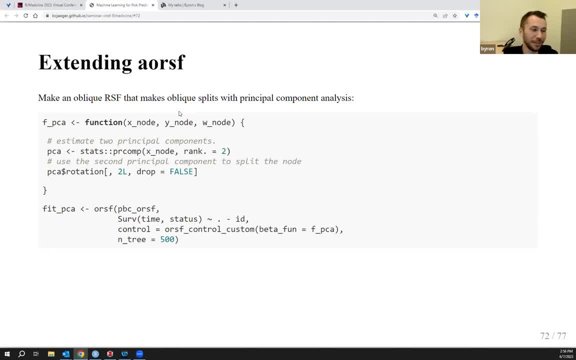 it's gonna cause your R session to crash. it won't be sent into C++. Instead, you should get back an error message that kind of says like: here's what it appears your function is doing. that is gonna cause the R session to crash. 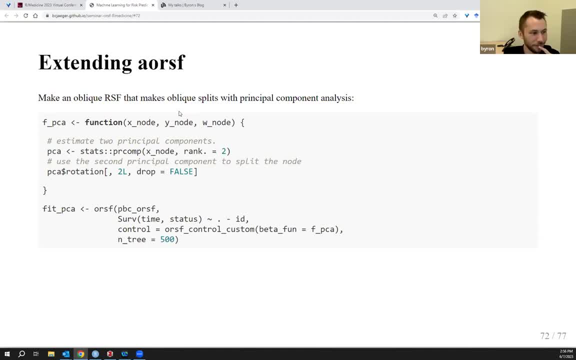 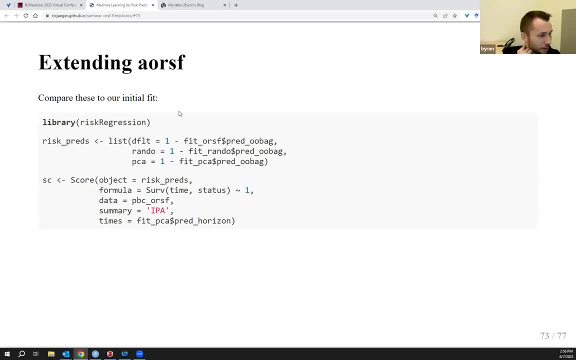 And so here's how you can hopefully modify it and make it work better. And I saw a little question in chat, so I'm just gonna read that real quick. I think there would be. So the question is: would there be a certain function to use? 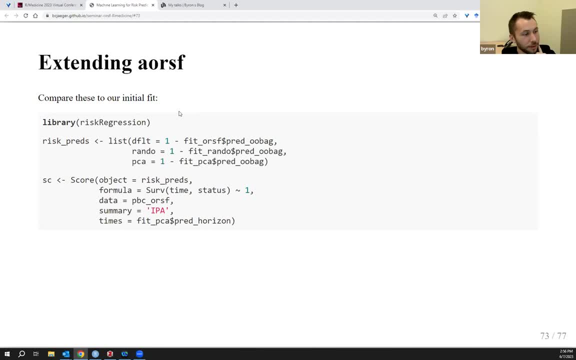 that would make a standard random survival forest, And there are a couple of ways that you might be able to get at that. So you could kind of just say: return a matrix where all the coefficients are zero except for one, And that would give you a standard random survival forest. 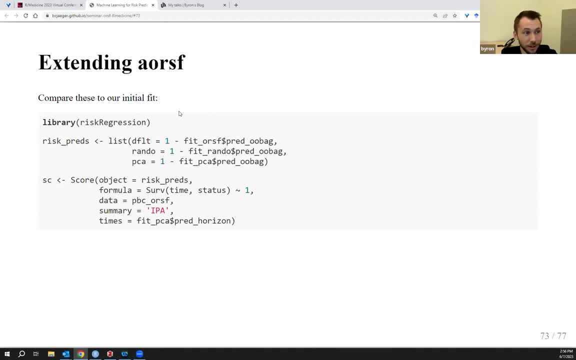 because you're just using a linear combination when you're removing some variables with that linear combination by multiplying them by zero. Or I think you could also fit the random, the oblique, random survival forest with a value of one for mtri, so that you're actually creating linear combinations. 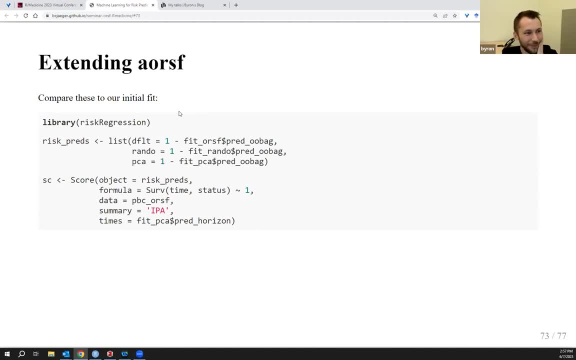 with variables, but there's only one variable. So it's like that's a trivial linear combination, but you would end up with something that looks a lot like an axis-based forest that way, And so great question. So now, if you ever wanna tune, 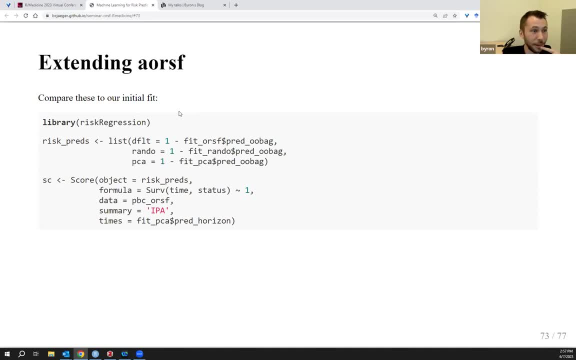 your random survival forest. this is kind of the way that I think about doing it, just by comparing the axes of the random survival forest. So let's say, I actually received the forest based off of its out-of-bag predictions, right? So here I've just got three different approaches. 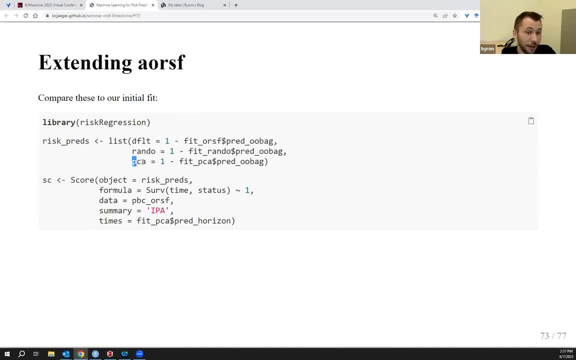 to fit this random survival forest. One is the default approach. One is using random coefficients. Another approach is to use principal component analysis And I'm pulling out the prediction, the out-of-bag predictions, from these three separate fits right. So I'm creating a list of risk predictions. 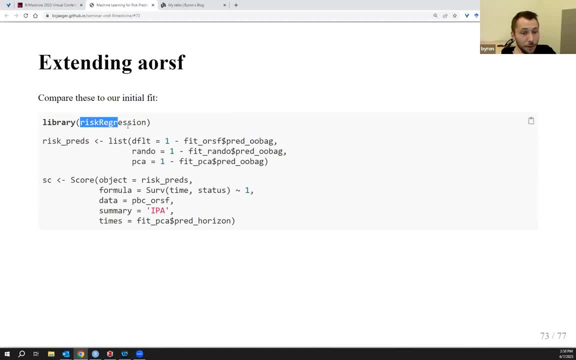 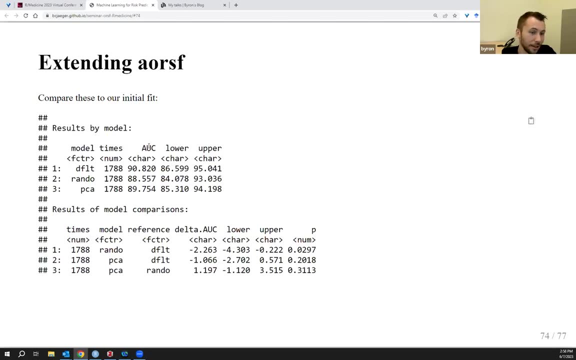 and then I pass that to the score function. so the risk regression package and it does a very nice job of evaluating accuracy of risk predictions, And so now you can just kind of get a look at how the three different approaches did. The default approach has an AUC of 90.8.. 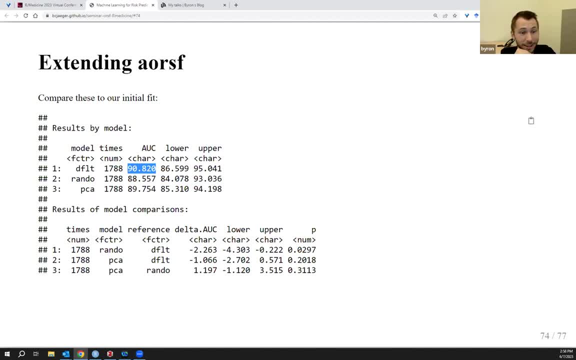 The other approaches do surprisingly well. I'm very surprised that you can just take some random coefficients and you get back a pretty good AUC. That's interesting to me. It's also interesting that this principal component, analysis, does almost as well as the approach. 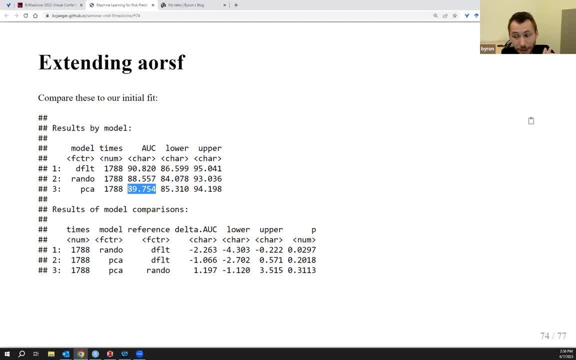 of using Cox regression. In fact, I don't have it on my slides, but there are a couple of data sets where the principal component, analysis, does better, So I'm very interested in what people may think of when it comes to you know. 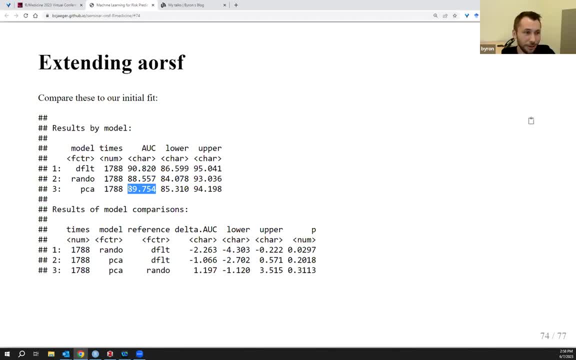 new ways to find linear combinations of predictors, because there is a good amount of variability in, like the performance of the opiate creative survival forest. that's explained by how you're actually computing the linear combinations. So thank you for sticking with us to the end. 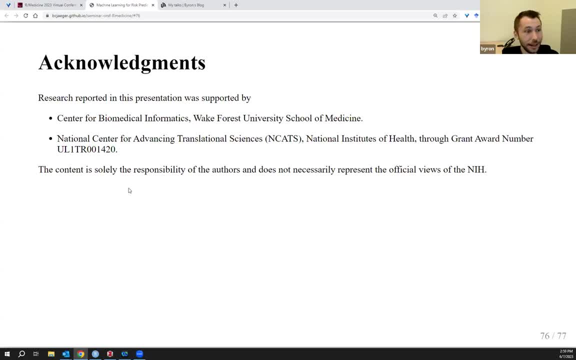 This is just a list of what we covered. I would like to acknowledge the funders of this research. It's been really nice to have some time to you know, support, a time to work on this And, of course, the collaborators who have helped along the way are all pictured here.